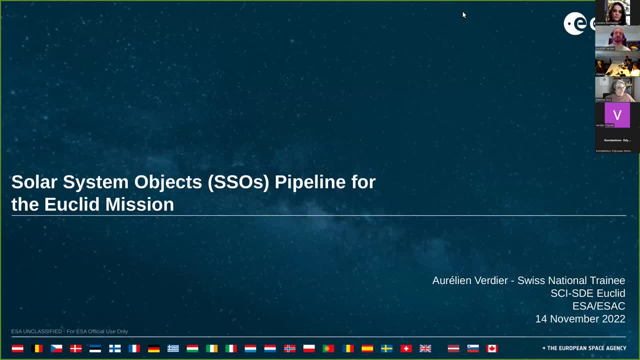 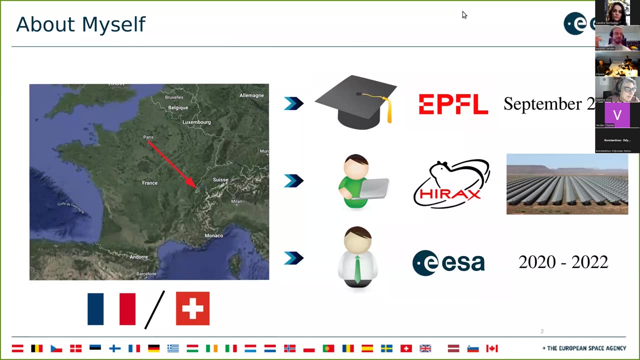 I'm currently a Swiss national trainee here in Madrid, so close to Madrid in Spain- And today I'm going to talk about the solar system object pipeline for the Euclid mission. So I already had a good presentation from Martin. but just to specify, my master work was about HIRAX. 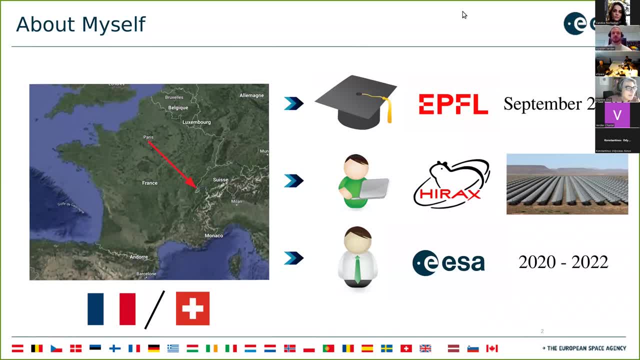 which is the one of the radio radio interferometer developed in South Africa, And so now I'm working. after this, I directly went for the national training program And now it's been two years, I'm here and my contract will end in two weeks. 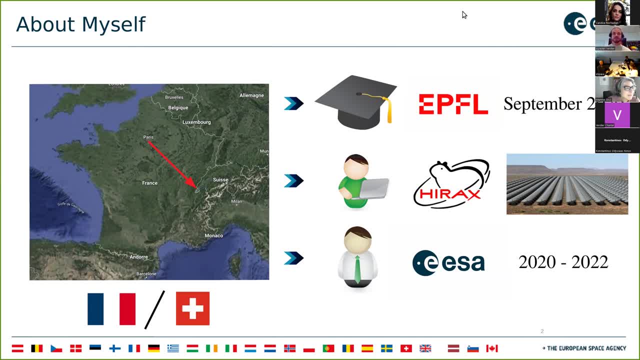 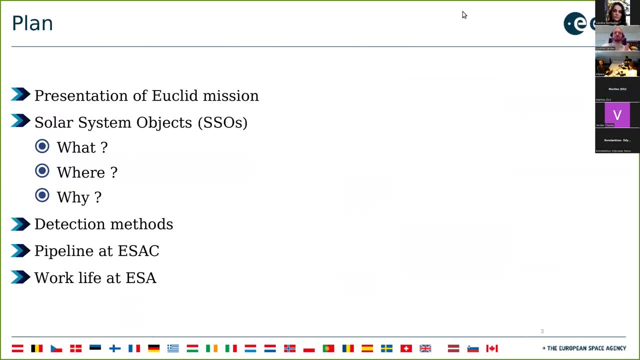 So it's kind of nice now to finish everything to show, to present you everything I could do for two years as a Swiss national trainee. So the small plan of the presentation. first I will present a bit the Euclid mission because I think 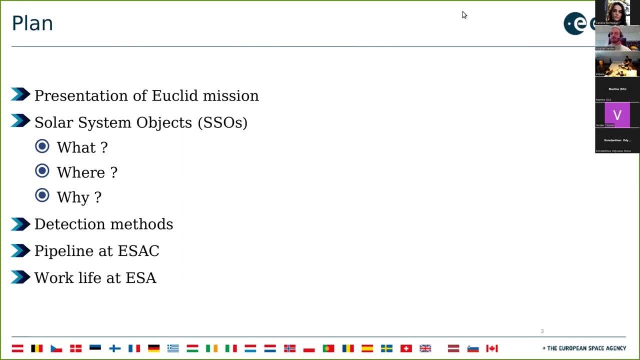 it's a marvelous mission and we need to talk about it. Then we'll talk about solar system objects- What are they, where are they and why do we need to detect them, Then talk about detection methods, Then the pipeline we're using here at ESAC to detect them, and then have a final list of SSOs. 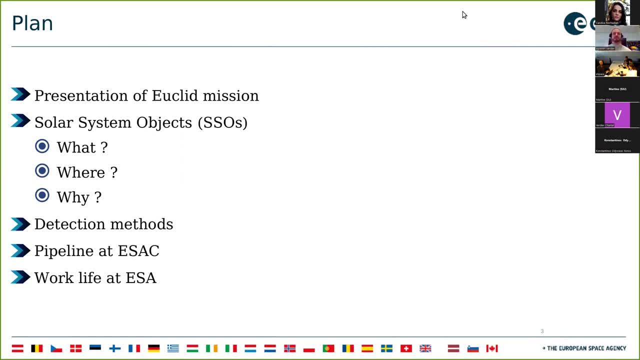 So you will hear me saying SSOs instead of solar objects all the time, because it's going to be kind of long, And then I'll talk a bit about the Euclid mission. And then I'll talk a bit about the Euclid mission. 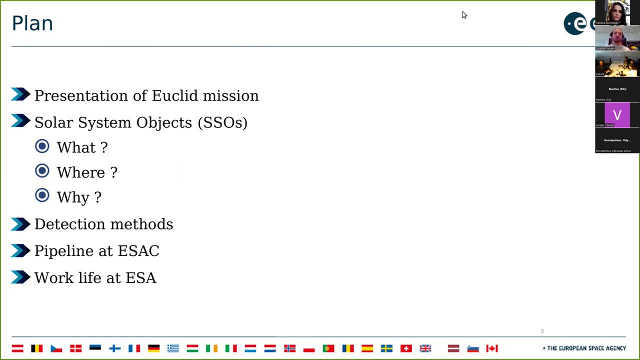 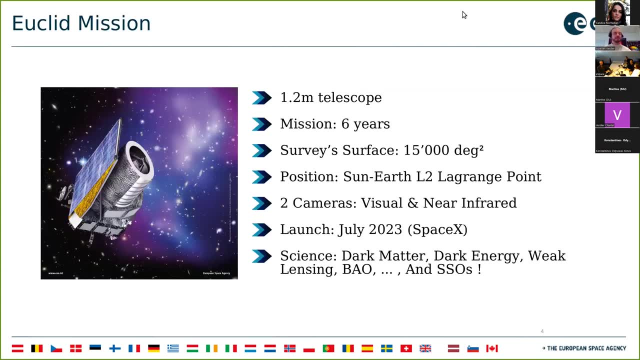 And then I'll talk a bit about the work life at ESA to make you maybe join the YGG program if you just finish your master and you're looking at this presentation, So let's go into it. So here is Euclid. It's a space mission. 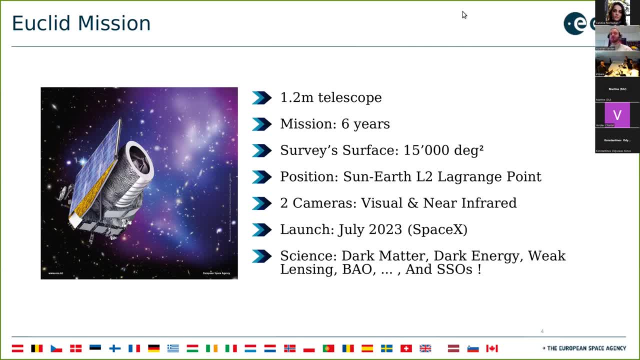 So it will be a telescope sent into space. It's a 1.2 meter mirror. It will be a six years mission And this is what we call a survey mission. So for six years we just map the sky And then at the end we will have: well, during the mission, at the end we will have 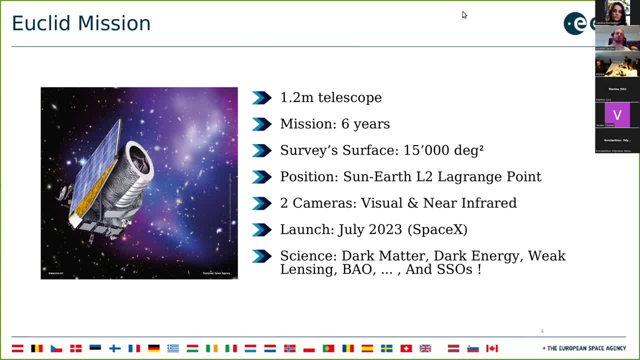 well during the mission at the end, we will have. well, during the mission at the end, we will have all the data available for anyone. The surface is 15,000 square degrees And it will be located in the Sun-Earth L2 Lagrange point. 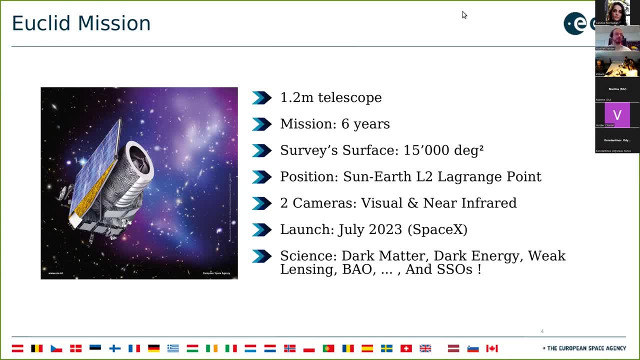 I will show you after this, for the people not knowing what are the Lagrange points. And there will be two instruments: First one for visual, which is this, and the second one for near infrared, which is NISP. The launch is now official. 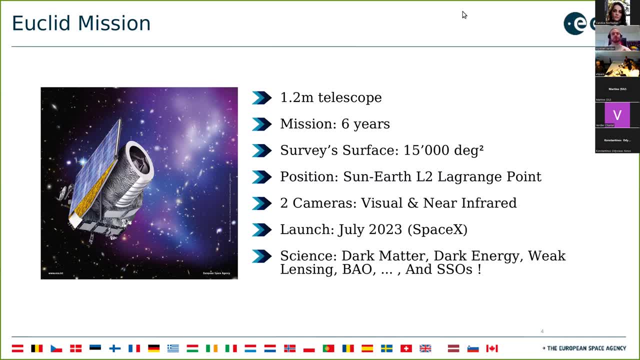 We had some trouble with the launch date And the launch will be in July 2023 with a SpaceX rocket. So finally we can launch Euclid, which is a very good news, And the science will be mainly dark matter, dark energy with weak lensing. 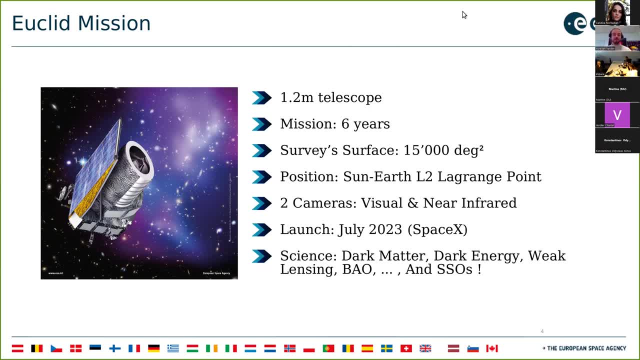 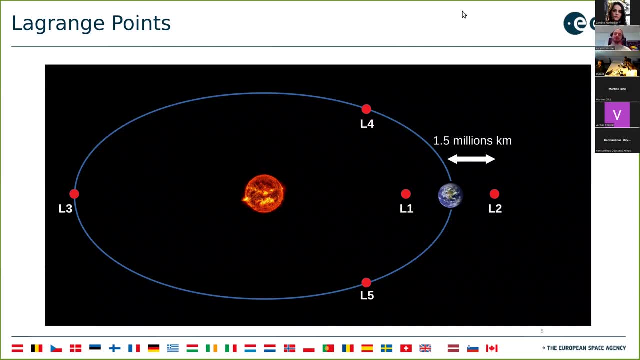 bionic acoustic oscillations and in between all of this we have SSOs. So yeah, just to show you where is the L2.. So maybe you know the GEMS Webb Space Telescope. it will be also be there. 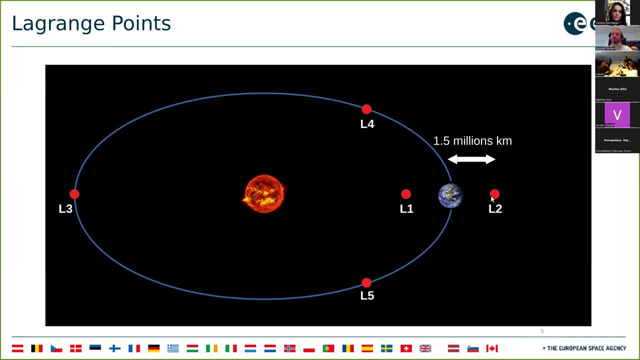 So, as you can see, the second point is here. It's a gravitational equilibrium in between Sun and Earth And we can send some space telescope there. They will stay. they will remain in this point. So it's kind of useful to send stuff there. 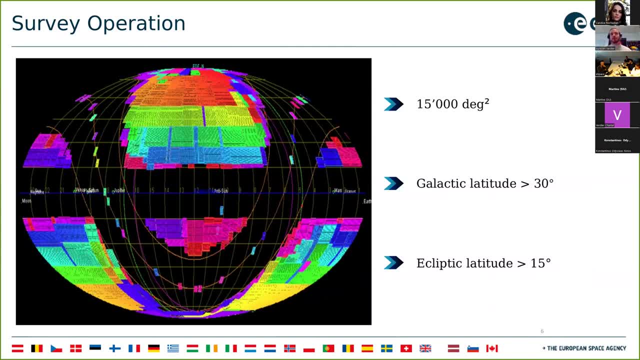 About the survey operation. Here is a picture to show you everything that Euclid will look at. So this is the whole sky You have to see like this is the whole sky and all the colorful squares means this is where Euclid will look at. 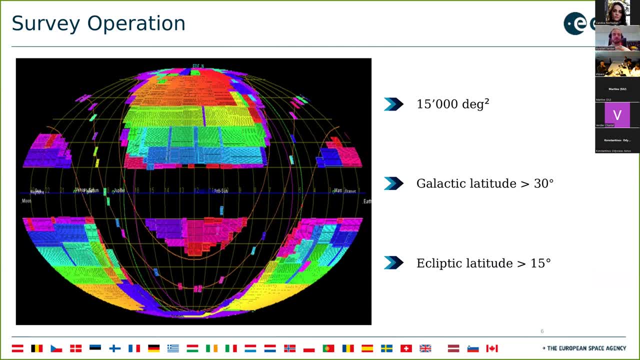 So you can see the dark matter. The dark spots are where we have. the ecliptic latitudes, so where the Sun and the planets are where our solar system is, and the galactic latitudes, so where is our galaxy? So, as we want to look at all the objects than our galaxy in our solar system, Euclid is made for this. 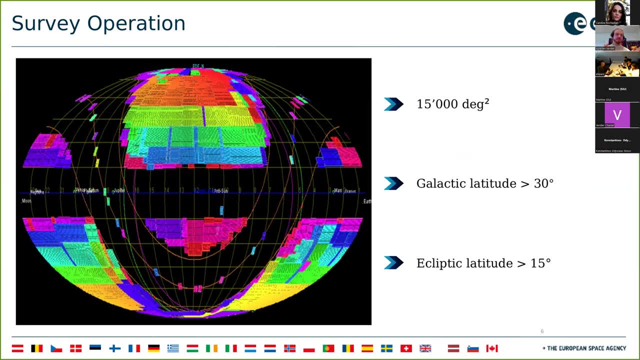 We don't look at this, We look outside those two objects. So this is what we will look at. I will ask you to remember this picture. We'll come to it later Because it's kind of important for Solar system objects. 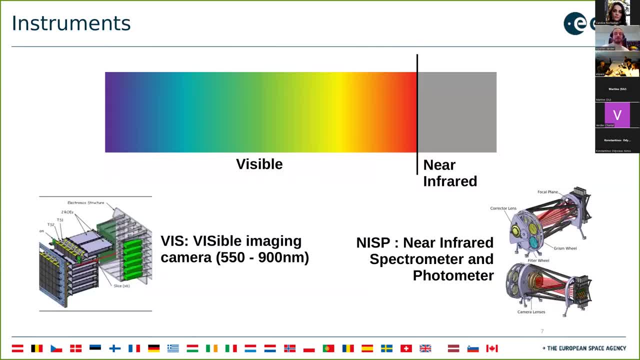 About the two cameras. So, as I said, there is two, There is this and NISP. So this is about visible. So, looking to the blue, red, yellow, red, like a Hubble did, And there is NISP, which is near infrared, just after the red. 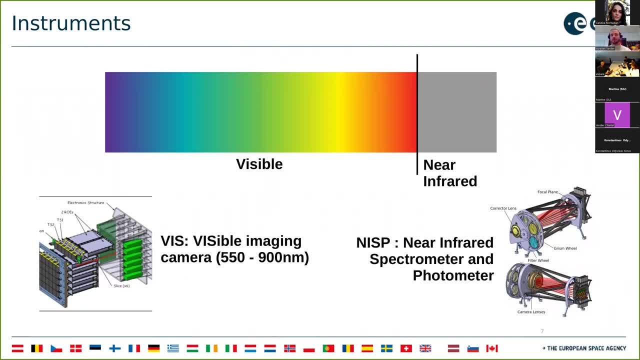 And it will be a spectrometer and the photometer. I've been mainly working on this data, So I'm not an expert in NISP. So sorry, if you have a specific question about NISP, I might not be the correct expert for this. 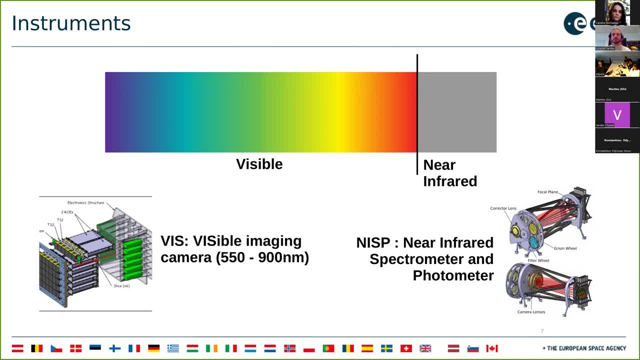 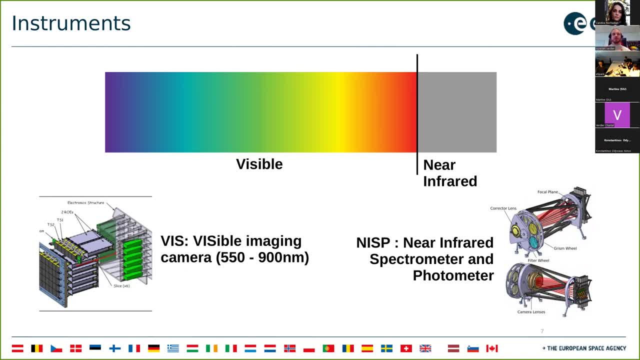 I'm not an expert in NISP, But I've been mainly working on this data, So I'm not an expert in NISP And I'm not an expert. So sorry, if you have a specific question about NISP, It might not be the correct expert for this. 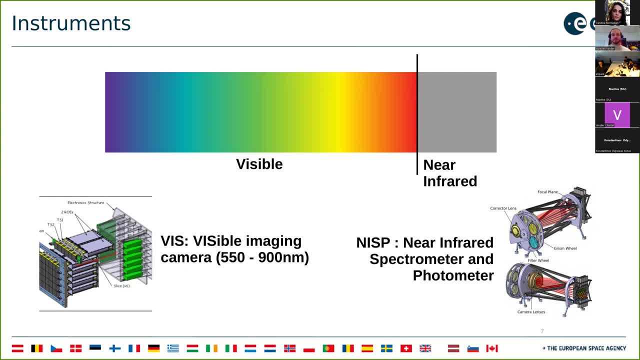 But I'm not an expert in NISP And I'm not an expert in NISP, The field of view of Euclid will be So for one picture of visual point, 57. Street, square, Square degrees And the true cameras. 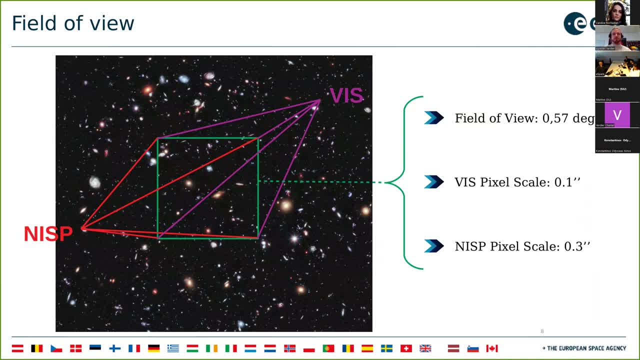 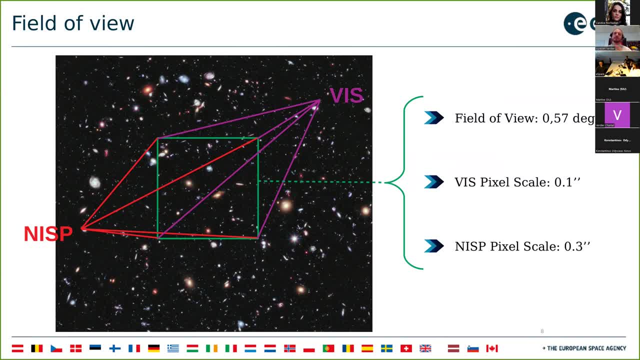 Uh Camera, Uh Camera. precision will say so. this is very precise with 0.1 arc. second, this piece is less, less precise, but as it is spectrometry, it's not a problem, and it will look like this. so the camera will be made. 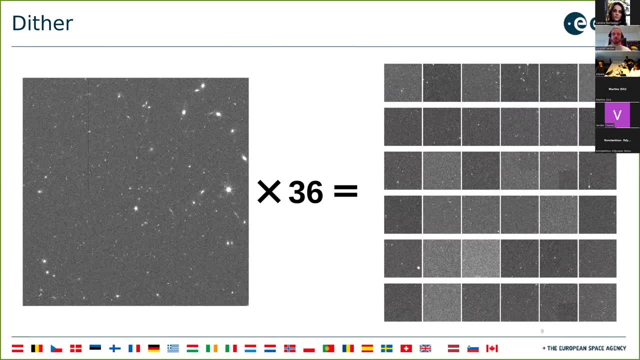 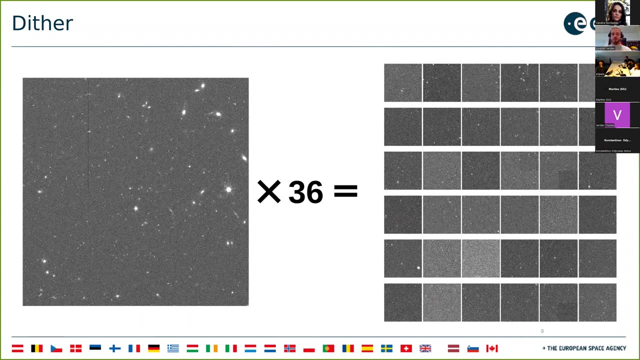 of 36 ccds. each ccd is 4000, around 4000 times 4000 pixels. so it's very huge. and even these ccds, then 36 ccds, so it's a lot of information in only one image, but it's not over. when we will be? 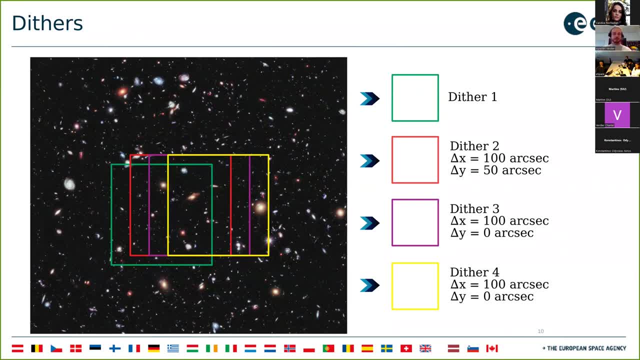 doing the mission, we will move a bit the camera, so there is what we call dithers. so the first dithers correspond to the first 36 ccds i showed you, and then there will be a small shift for the second dither, and again another shift and another shift for the remaining ones, just to fill the gap. 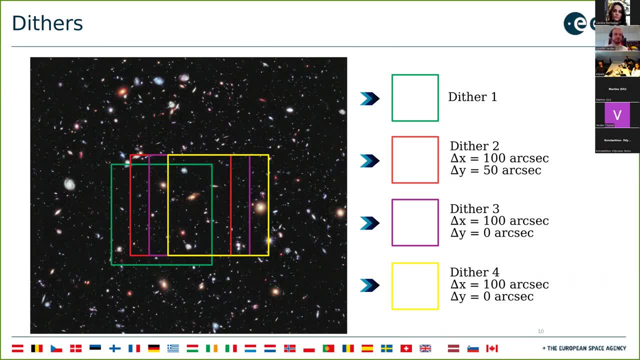 in between the ccds. so at the end we get a beautiful picture of the ccds and then we have a beautiful picture of the ccds, and then we have a beautiful picture of the ccds and then we have a picture without any holes. for euclid, unfortunately, we still haven't any picture. 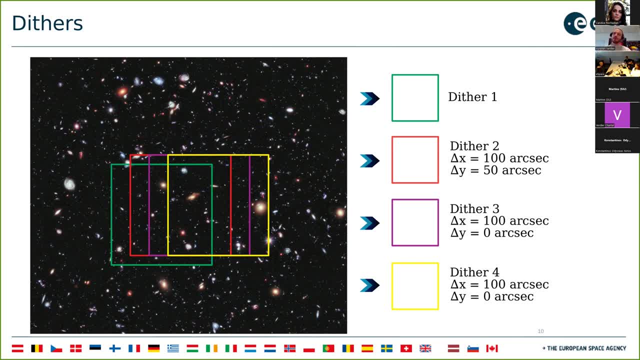 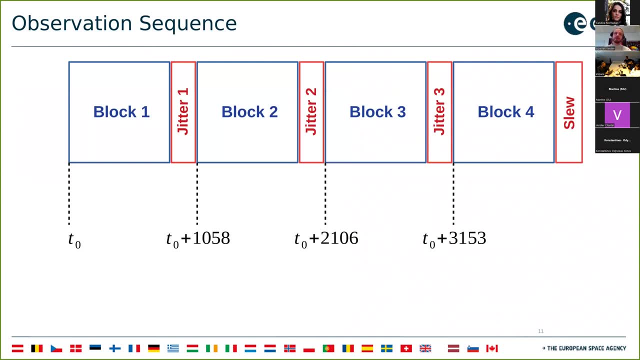 because the spacecraft is still on earth so i won't be able to show you beautiful pictures like hubble or the gems web. we will have to be patient to to see those kind of pictures. the observation sequence. so how will what we will do in each dither so it's separated in different? 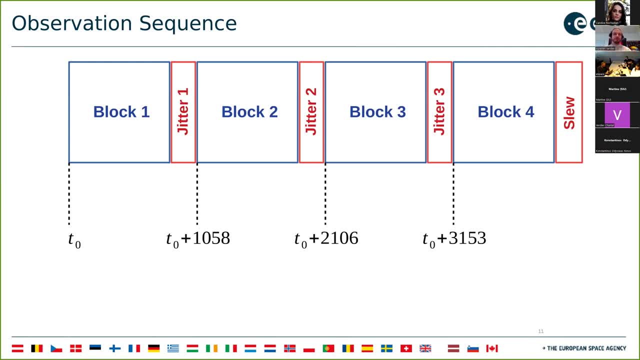 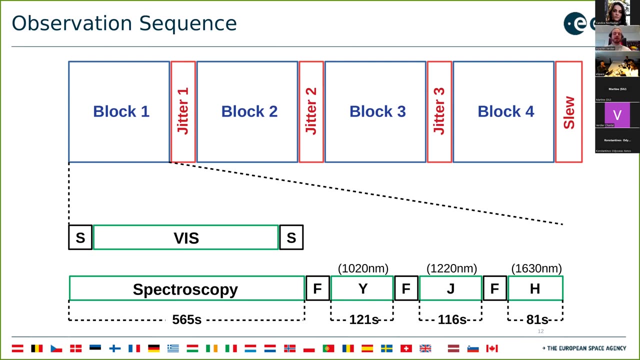 blocks. so block one corresponds to dither one, block two to dither two and so on, and each block will be separated by around 1000 seconds. during those 1000 seconds, a lot of stuff will happen in parallel. we will have this starting to take a picture and we will have nisp starting to. 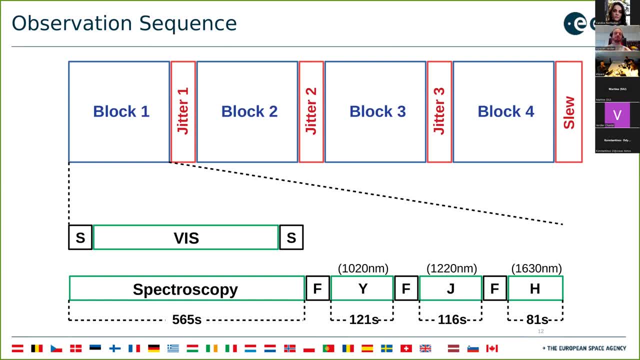 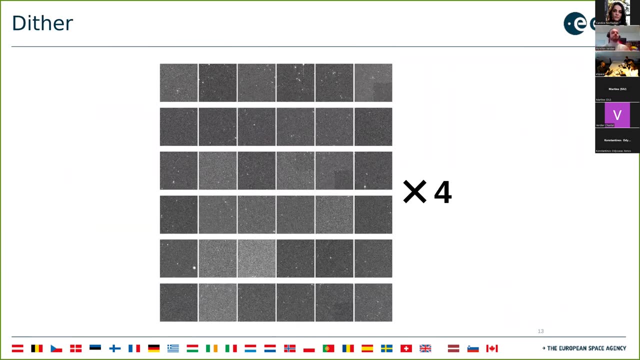 do the spectroscopy and then, after this, use a near infrared filter. so they are named y, j and h, and they will proceed to do some pictures too. so everything will happen for each dither. so at the end we have this picture times four. so, as you can see, we will have a lot, a lot and a lot of information in only one picture. 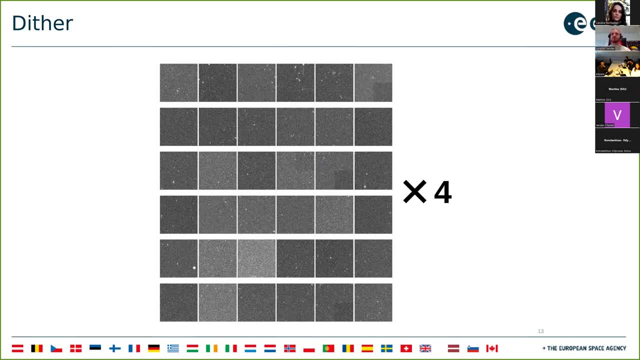 so this is the. the main reason euclid has been saying is to have a wide information about space. for example, if we come back to gems web, it's about having deep information, very precise information. with euclid we'll have wide um wide information. so where let's see how they are located and stuff. 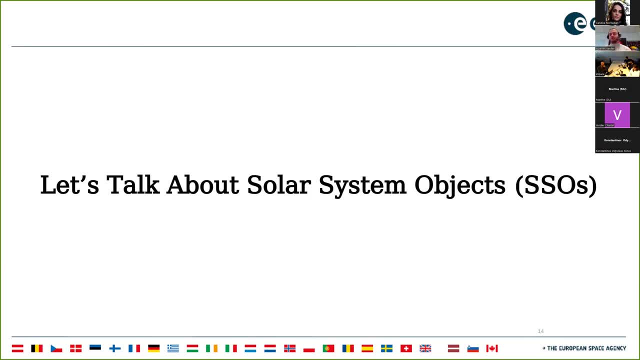 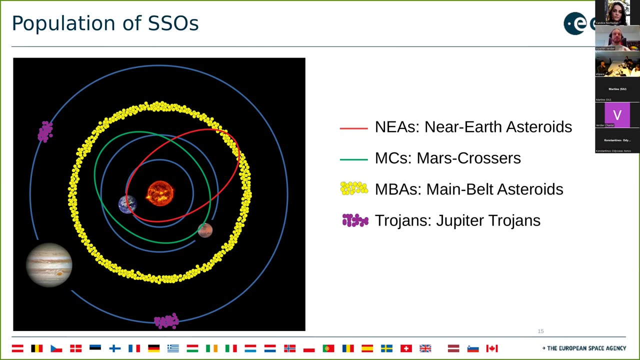 like this. so this was about euclid in general, and now i would like to speak about my work, which is about solar system objects. so what are they? it's another name to just say asteroids, but maybe we will find other objects than asteroids, so maybe we still have the name solar system objects to mean. it means 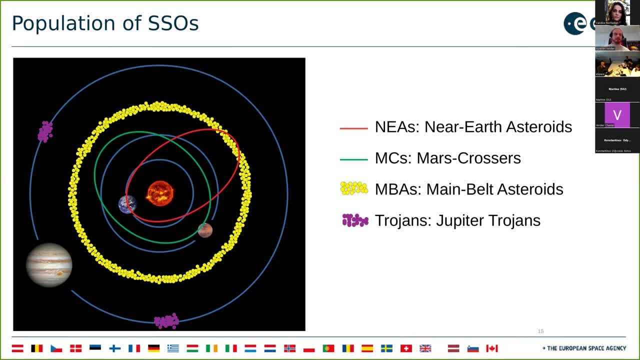 that it's objects located in the solar system. so we are looking at very close objects with a spacecraft that is supposed to see objects very far away. i will come to that later. so where are those? uh asteroids or ssos? so of course we have some close to uh earth with the 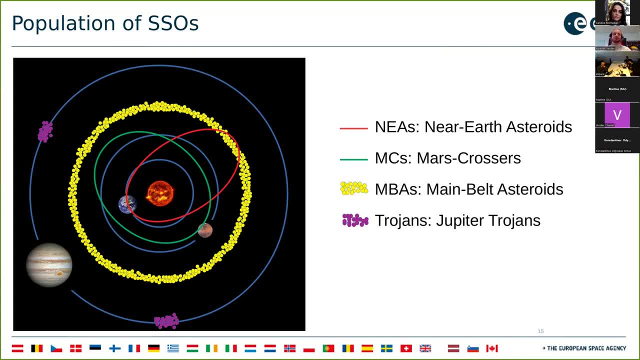 near-earth asteroids or to mars with mars crossers. you should know, i think, from school that we have the main build asteroids just in between mars and jupiter. we have some- i don't know, i like i think it's kind of funny to have this- asteroids just on jupiter orbits that are a bit stuck there because 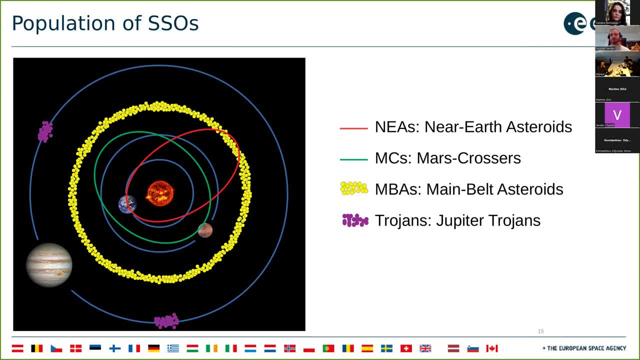 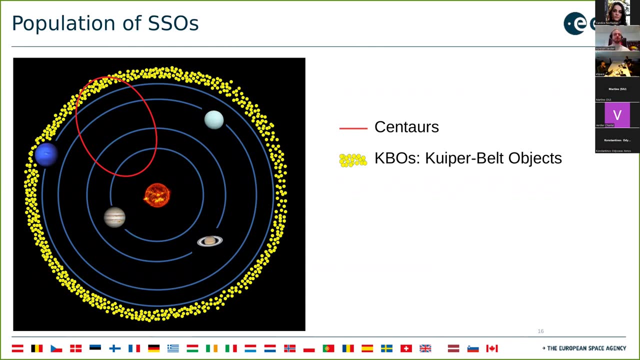 jupiter in uh and um and uh the the sun has have also some of the asteroids that are stuck there, the lagrange point. so you have some uh stuck asteroids just there and even further. we have also again asteroids just going to the jupiter orbit and we have this creeper belt object, which 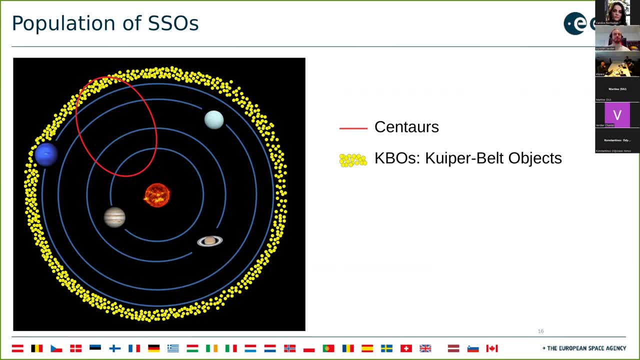 is kind of the same as the, the other belt, but behind neptune. so a lot of objects to detect there and we still have a lot of work and a lot of information uh to to to have from them. now the question is: okay, we have those uh. 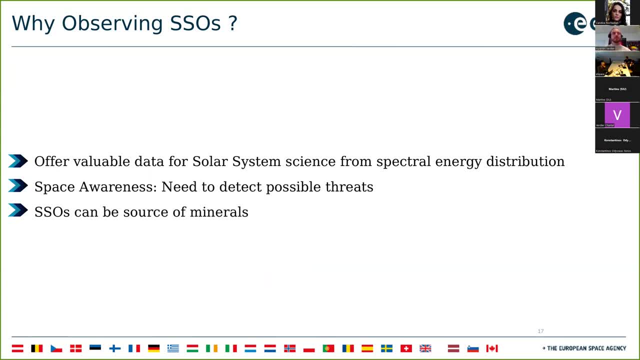 rocks around us, but is it very important to watch them or not? uh well, there is three main arguments to say we need to detect them and to observe them. the first one is that they are the relic, like a historic part, of our solar system and its evolution. so if we want to have information about 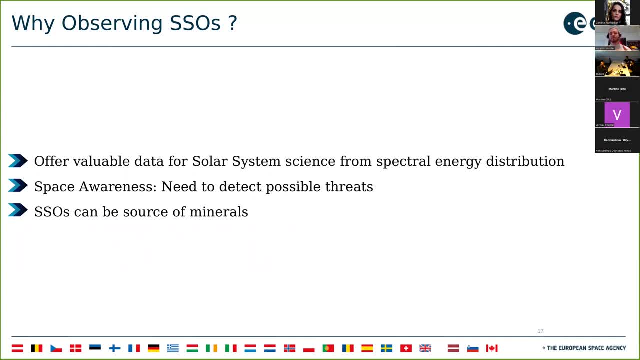 how the solar system was created and how it evolved. we can find those information with the asteroids. the second point which is, i think, very important for every one of us, is the space awareness. we need to know if an asteroid will come to earth or not and if it's dangerous or not. and the third one is maybe later for the future- is that there is a lot. 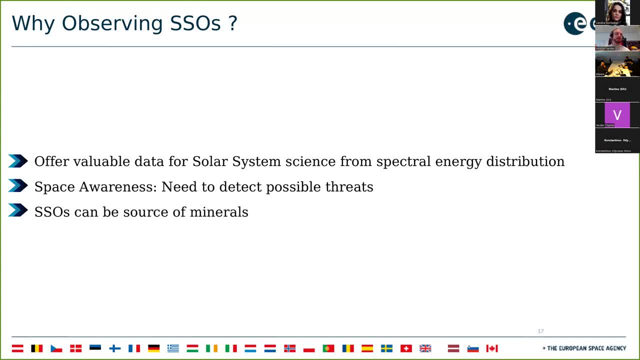 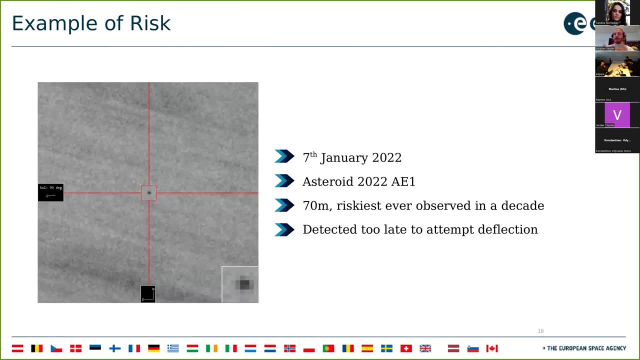 of stuff in in the sso, so maybe we can like just mine them later and have more resources for for us on earth. um, i want to come back about a risk because, for example, this year, um, it has been announced that we were kind of lucky because one asteroid was detected as a big risk for earth and the problem was that it was a 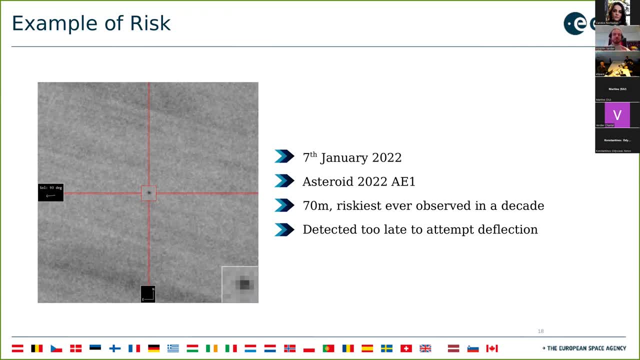 bit hidden by the moon. so they had to wait for a month to have more information to know if we were gonna have a big problem. not, and at the end, a month later, they were like, oh, don't worry. uh, we did not tell you there was an asteroid coming, but finally it would just pass close to the earth. but 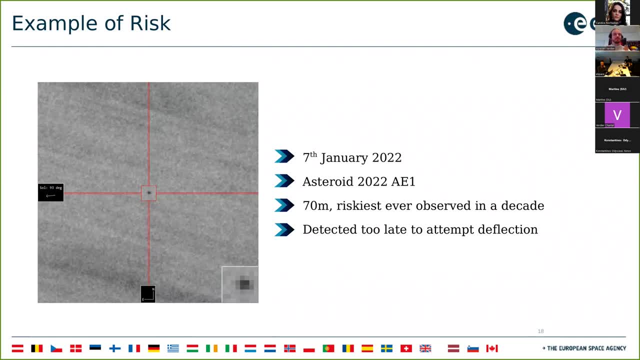 not on us, so good thing. but, as you can see, this one was detected so lately that had no, no, no issue. like we, we could not, uh, attempt to deflect it. it was not possible, it was over. so we really need to know what is around us. nasa is already doing it quite well, but 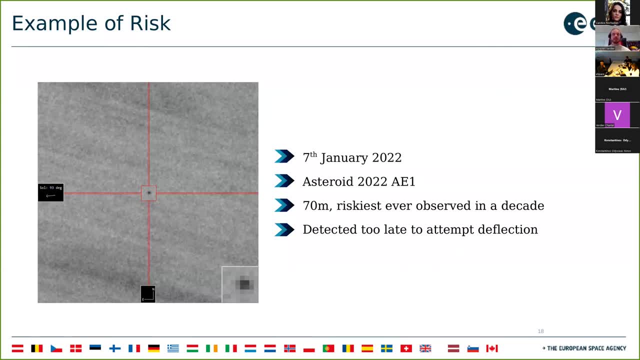 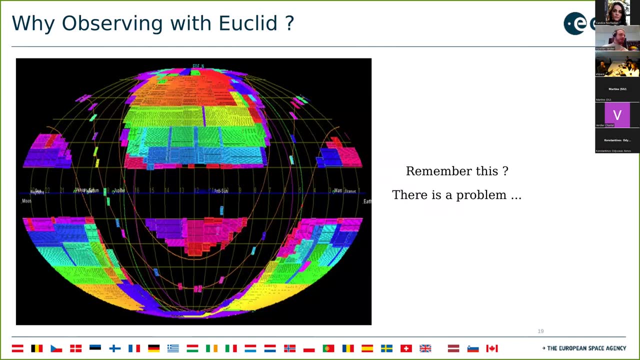 even with this, we still need more information. so the more asteroids mission we do, the better it is for us. um, so now, why euclid? as i told you, euclid is mostly a mission that will do deep space stuff that are outside our galaxy, in our solar system. and also, i asked you to remember this picture, and there is one. 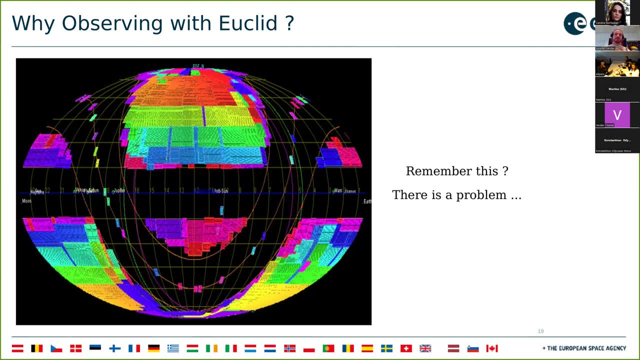 problem, uh, with uh, asteroids, with this is that it avoids the galactic plane, uh, the ecliptic plane. sorry, big mistake there. and the ecliptic plane is there, is where there is the solar system and the asteroids are inside the solar system. so can we really detect asteroids when we avoid the solar 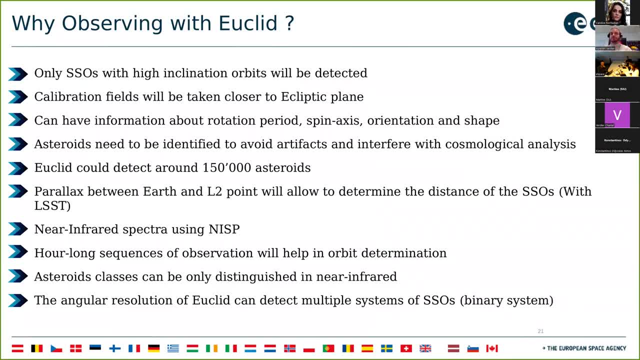 system with euclid? well, the answer is yes. um, the only ssos we will detect is high inclination orbits, because of course there is asteroids going around the solar system, but, you know, like going a bit up and down, not not following the planets and stuff. so it's good information to have too, because it's not necessary as there is. 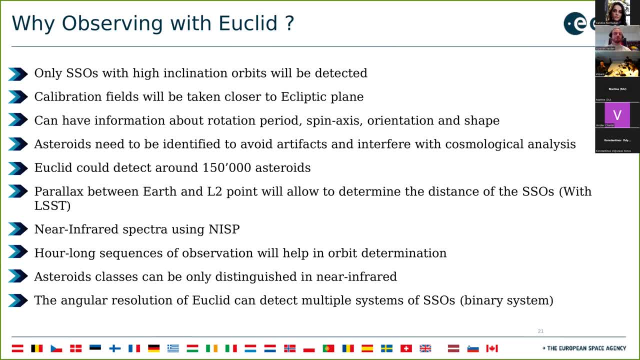 we look at normally. so maybe we'll have new objects, we don't know, maybe some stuff can be discovered via the euclid images. um, also, we might be able to detect some in the ecliptic plane, because, uh, for the calibration field. so when euclid will be sent, we will first 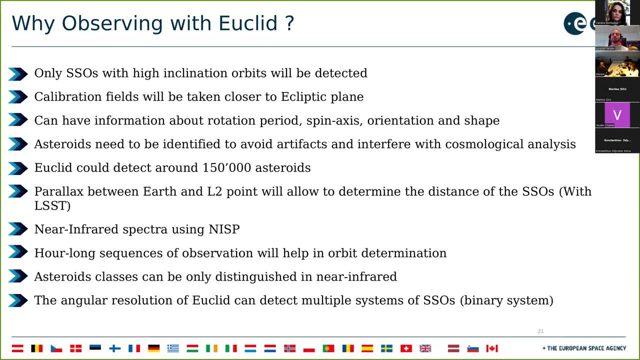 do pictures to see if everything is working accordingly and it will be indicated in the ecliptic plane so we will be able to detect, maybe, asteroids in the calibration fields. but euclid also is very precise, so we will have a lot of information about asteroids. so, for example, rotation period, spin axis, orientation, shape, um, also a little later. 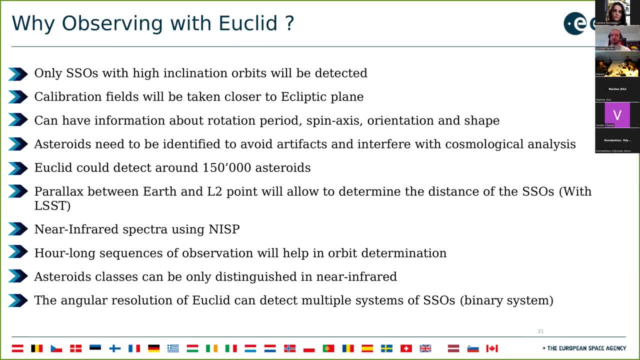 But as we will have NISP, NISP is in infrared And, from a paper sent a few years ago, asteroids can be classified only if we use near infrared. So we have the visual of the asteroid and also the near infrared at the same moment. 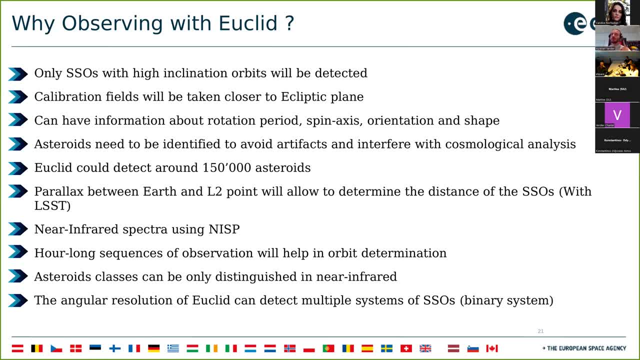 So it's very nice to have all this information in one mission. Remember that Euclid was not made for SSOs at all. It was only for cosmology. So it's just like someone saw what Euclid was about to do and he was like, okay, well, we have anything we need for asteroids. 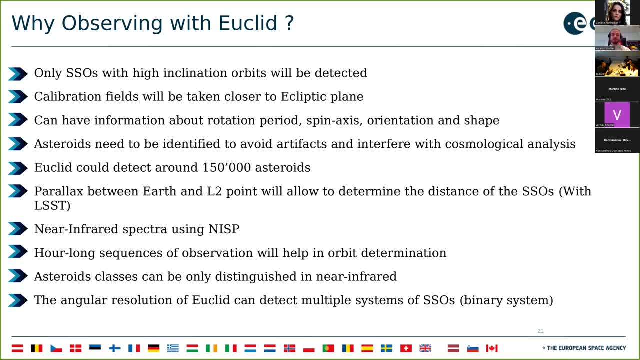 so let's do it. So it's a parallel mission, And now we want to do it with Euclid, Also for cosmology, as Euclid is using cosmology. knowing where are the asteroids in the pictures means that we will have less noise inside the pictures. 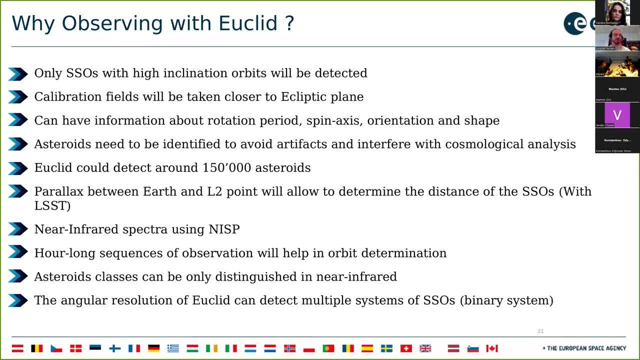 which is nice for cosmology. So also it's nice to detect only for Euclid. We will have around 150,000 asteroids, which is still a huge amount of detection, So it's good for science And as Euclid will be in the L2 point, 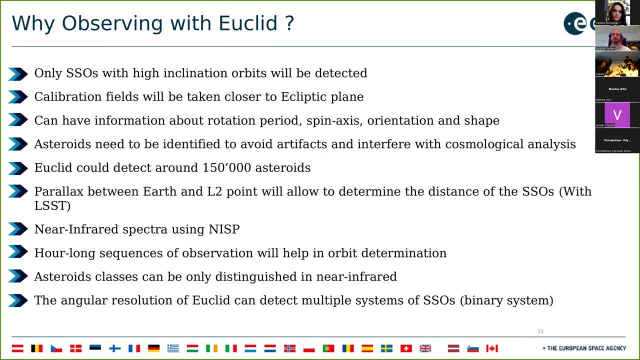 if we do observation at the same time, from what will be the case with the LCCD mission, then we'll be able to have the exact distance of the SSOs with using the parallax. Also, we have how long sequences. So with the distance and this, 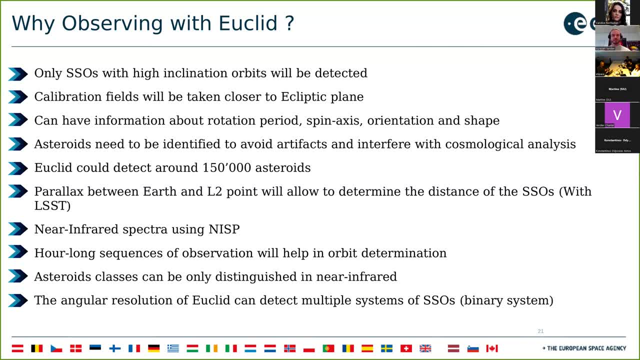 we can have a good information about the orbit of each SSOs, which is what we want In case of. we want to send an alert for Earth. So more information about the position and the orbit of the asteroid, And also, apparently, Euclid, is very precise. 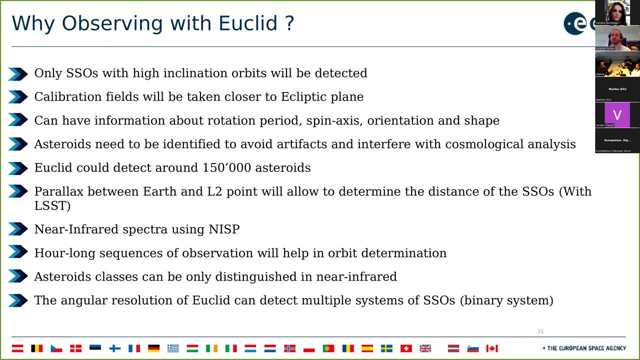 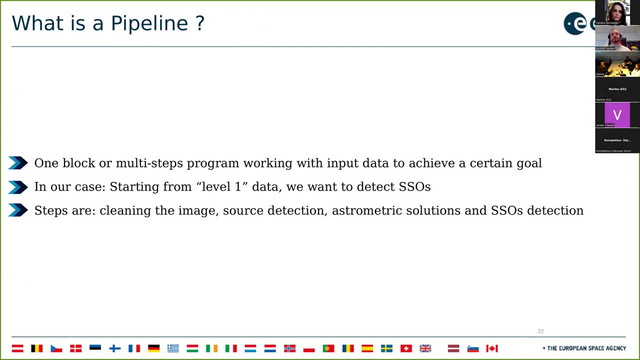 So we can maybe detect multiple system of SSOs. So that's also a good plus for this. So a lot of reason to do it. but now we need to develop what we call the pipeline to do it. So a pipeline, in our case, will be like a block. 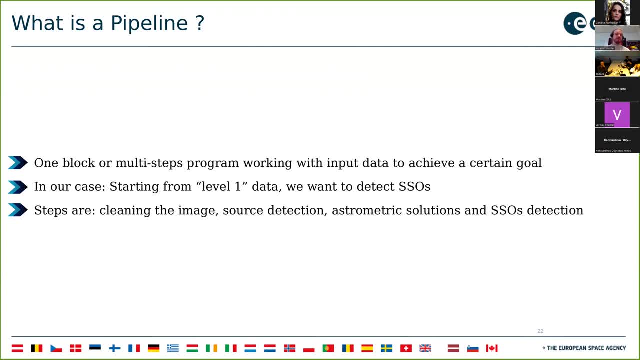 or multi-steps program that start from input data to the system. So we need to have to achieve a certain goal. In our case we start from level one data. We call level one data not the raw data, but just data that have been. 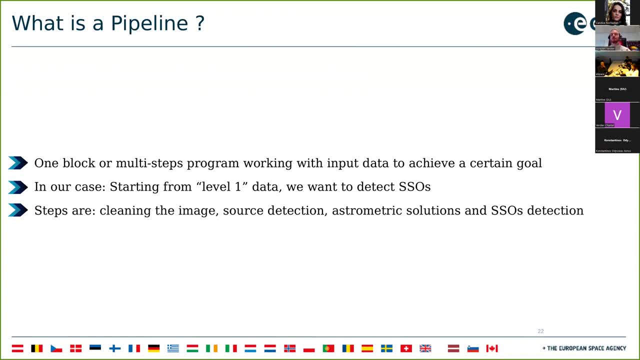 that can be used for science but are not yet cleaned- perfectly cleaned. Why we won't wait for clean data? Because, as I said, we want to send alerts very quickly. So if we detect an asteroid that might be a threat, we need to know the information as fast as possible. 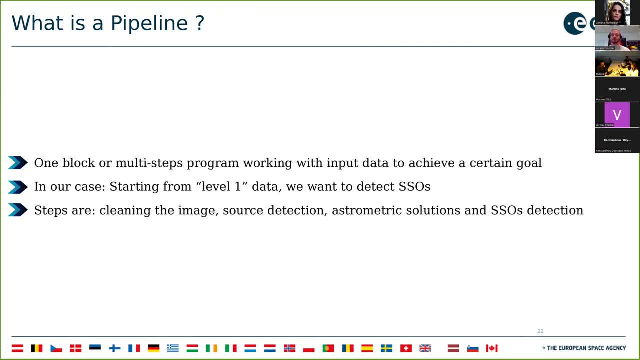 We cannot just wait two days to have the information, So we need to start from level one data and develop a quick pipeline to detect asteroids. So less than 20 minutes In our case. we'll have a multi-steps pipeline and the pipeline, what we call pipeline stages. 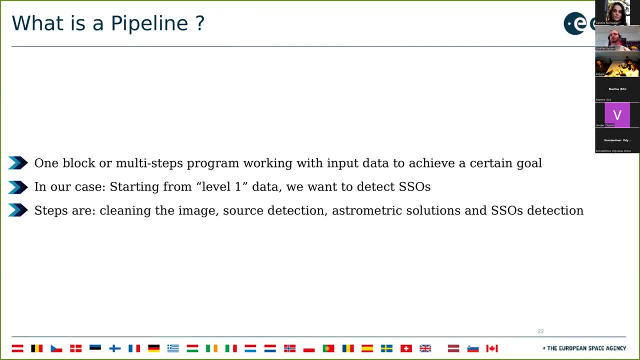 will be, for example, one for cleaning the image, one for source detection, one other for astrometric solutions. So we'll come to that later, And at the end we need a page for the detection of the SSOs. 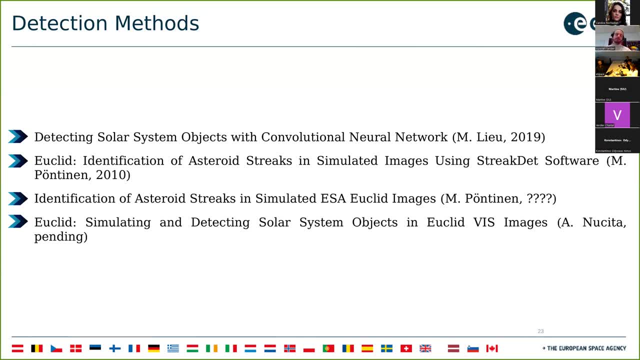 So to organize the pipeline you need to have a detection method and then you organize your pipeline around the detection method. There have been a few developed the last years around the project of Euclid, And I will present you all of them, So I'm not an expert in each one, of course. 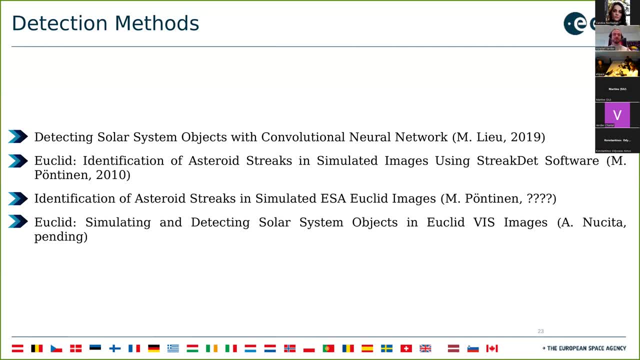 because I was not working into them. I had to read papers and to discuss with these people to understand what they were doing. But I think it's interesting to see what is developed within ESA And with other universities and other labs to achieve this goal of observing SSOs. 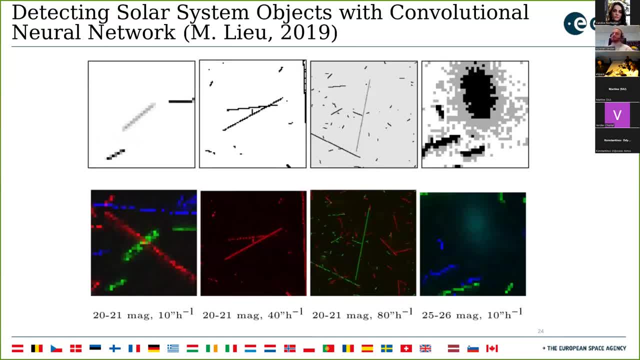 with a mission that is not made for this. So the first one of course nowadays is to use machine learning and the very well-known convolutional neural network. So in this paper the purpose was kind of simple. Normally, for example, with convolutional network, 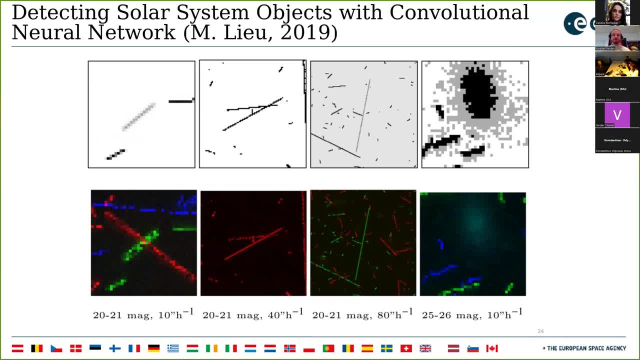 what you do is, if you have cat and dogs, pictures of cat and dogs, the CNN, so the convolutional neural network, will be able to say: whenever it's a dog, whenever it's a cat. Here it's kind of the same question is. 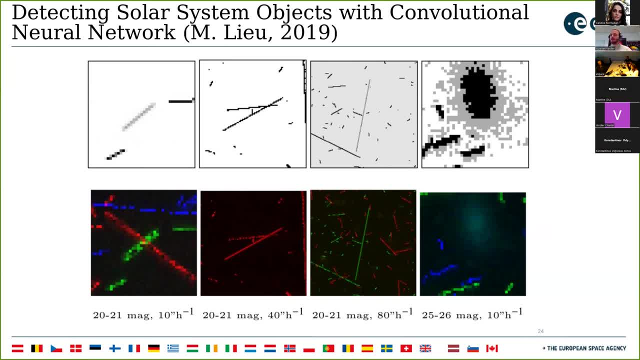 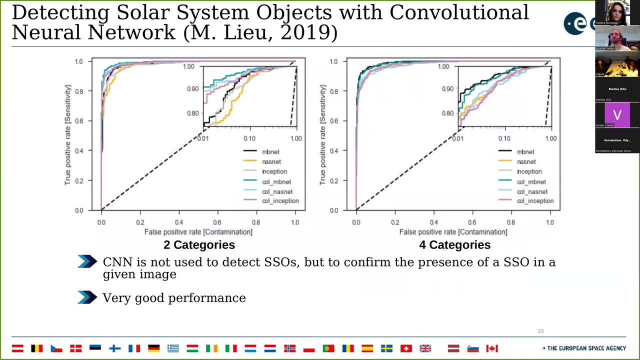 is there an SSO image or not? So in this paper, this is what they do. They have a lot of pictures with and without SSOs. They train the machine learning algorithm And at the end they get those results which are very, very good. 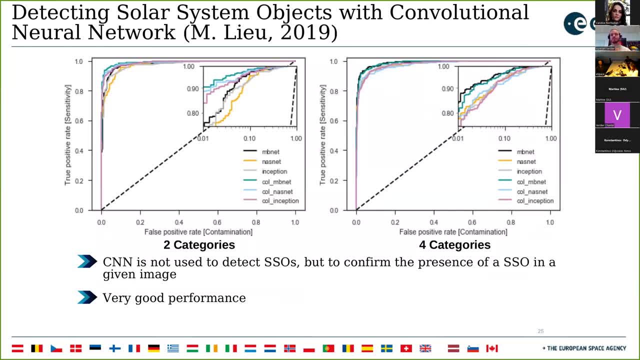 It's a very good performance. It's very easy to detect an SSO or not in a picture. Only one issue is that it confirms whether or not there is an SSO in the image, but it does not directly detect the SSO. 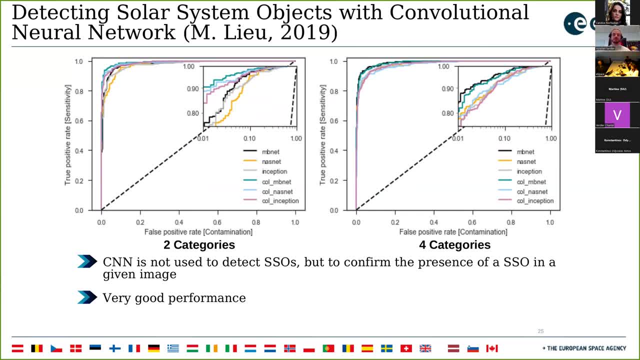 So if we provide a small picture with an SSO, then the machine learning algorithm will say: oh, yes, there is one here, but we don't have any more information. So it's basic information, which is nice. It shows that CNN can be a tool. 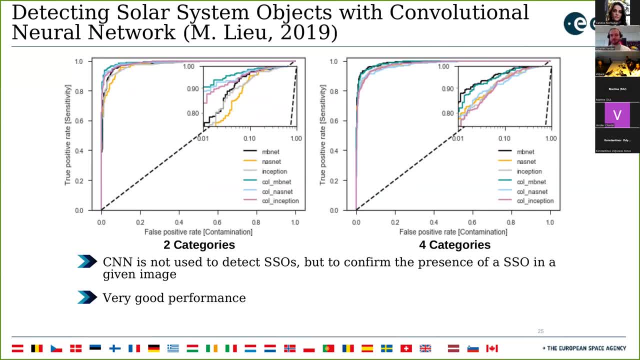 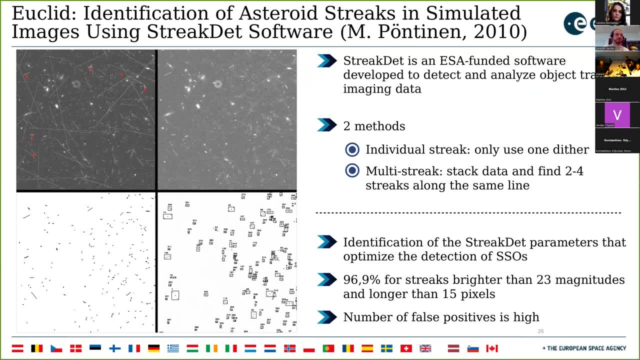 but we need more for the mission. but it's a first step. So another thing that was developed- I'm sure people from e-space know this one- because of space awareness. So we use normally STRIK-DET to detect satellites around the Earth. 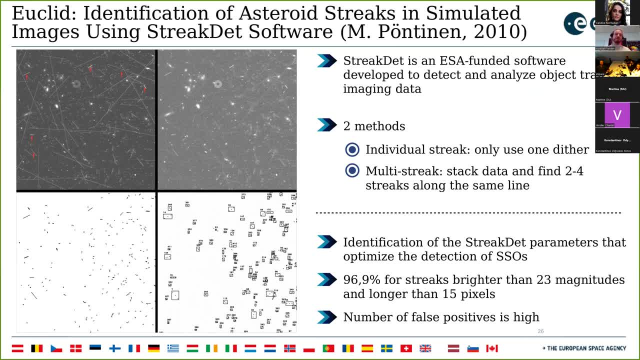 And so the question was: can we also use that on Euclid data to detect SSOs? So in this paper, this is what they did, And the results are yes and no. So for specific asteroids it works. So for bright asteroids. 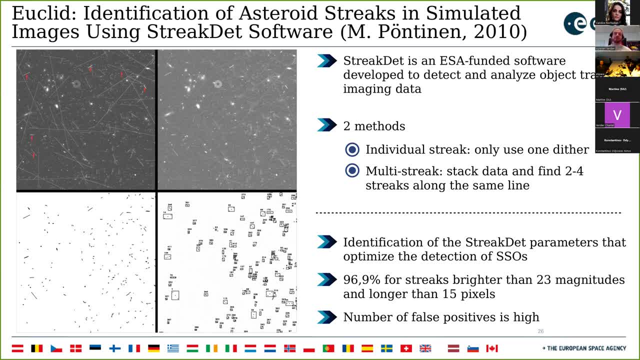 with a very long STRIK. it works perfectly fine. Like you can see, 96.9% of this. However, it's very specific And in general, it's closer to 60% of detection And there is a lot of false positive. 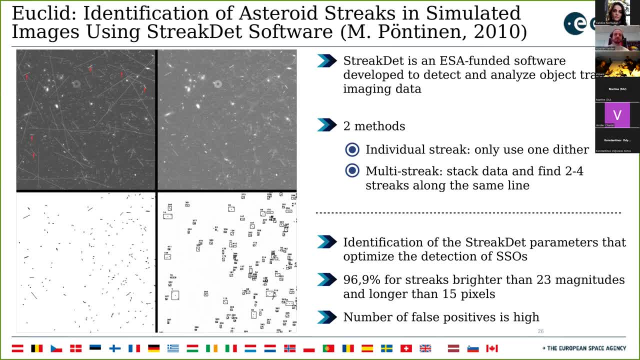 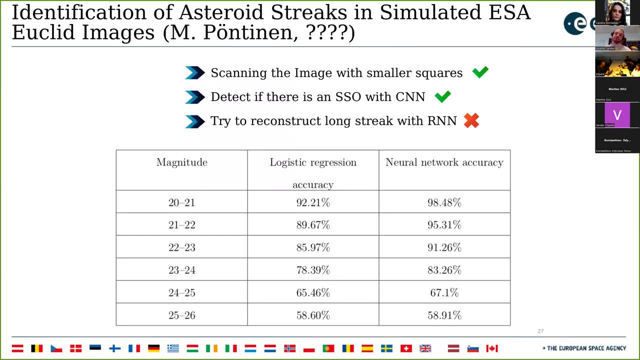 So the STRIK-DET is nice, but it's not enough for our mission, So we need to find something else. So now we go back again to CNN, But this time they want to do a whole pipeline using only machine learning to also detect and recognize the STRIKs of the SSOs. 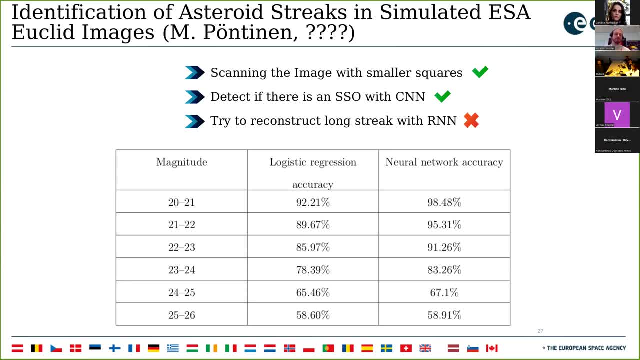 So, as before, the solution they use is just to analyze the image like small part per small part, for example 10 pixel by 10 pixel. So you scan the image like this and then you check in each little picture if you have an SSO or not. 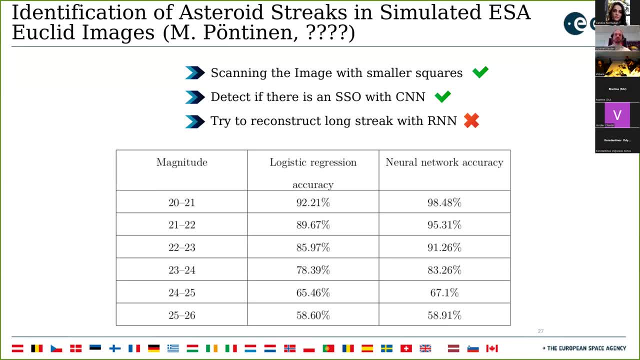 because you cannot just send the whole picture inside the machine learning As I showed you. it's, It's enormous, It's a huge amount of data. So you cannot just throw this into a machine learning program and say, well, do the work. 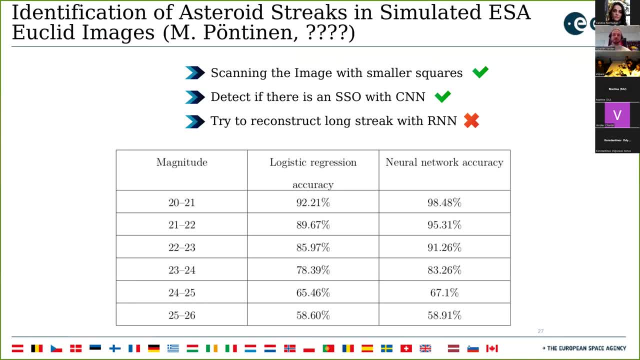 It cannot be like this, So you have to use smaller part of the image, one by one, and then detect if there is an SSO or not. This is perfectly working as it was before, But now the problem is that STRIKs can be detected multiple times. 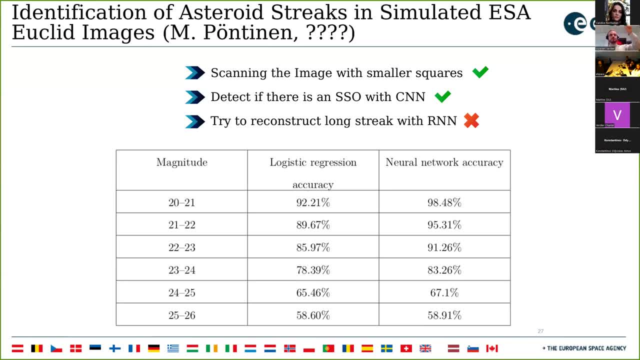 For example, if there is one STRIK starting in top left and just on the right is still the same STRIK, how do you tell the program that it's still the same STRIK? So for this they use the RNN algorithm. 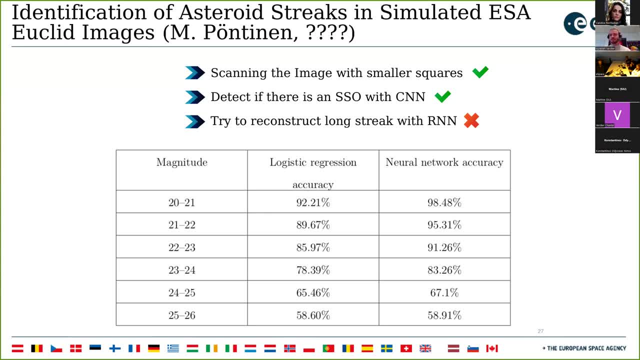 So RNN is normally used, for example, to complete one of your sentences. For example, if you say hello, my name is Well name, it's not working. but to complete the sentence you can use RNN. 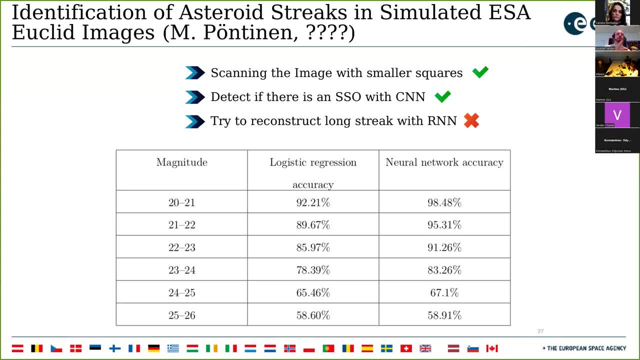 So they try to use like: because you have this information before in this image, maybe you can say that this information is the same. So they were working on this and the result is not very good. For now they are around 60% again. 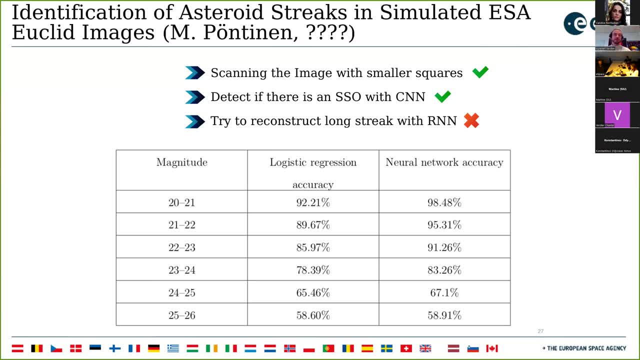 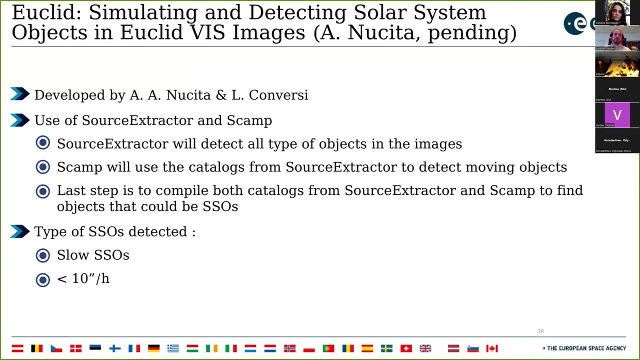 So still some improvement to do. I don't know where they are now, because last time we talked about this it was a few months ago And well, we have no news, So maybe it's not working very well. So now we come to the detection armor at ISA. 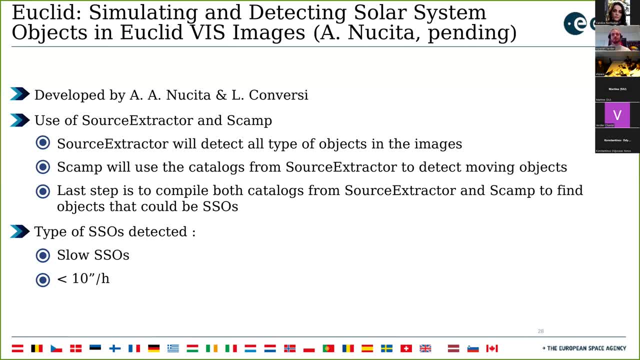 which use the more classical software from astrophysics and astronomy, which are Source Extractor and SCAMP. So SCAMP is also made by the same author of Source Extractor, And Source Extractor is very well known because it just extracts sources from images. 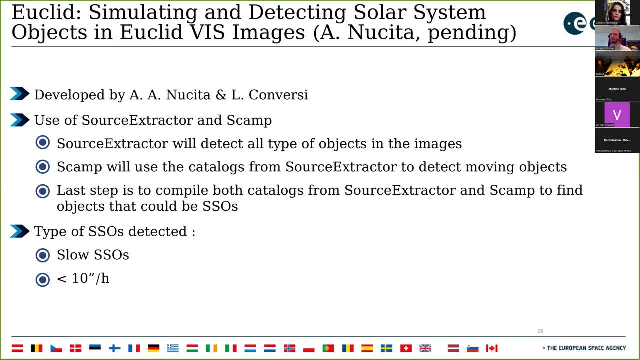 It's been used in every space mission. we know It's a very powerful software. So we use Source Extractor to detect images, We use SCAMP to align the images, So using the result of Source Extractor to align images, And then we try to find which objects are SSOs in the catalogs and which are not. 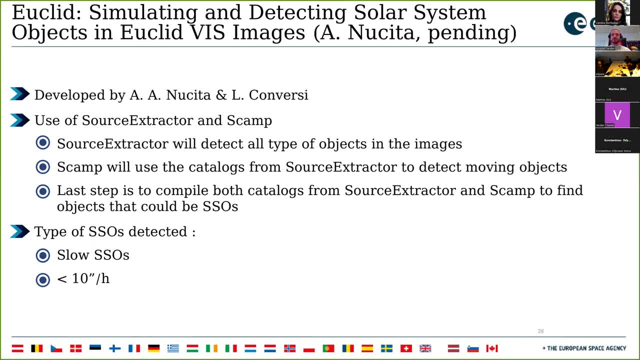 In our pipeline. which is important to know too, is that we focus on very slow SSOs, which means that the streaks will be very, very, very small Instead of the streak we saw before. CNN is very nice for this and maybe other software for very long streaks. 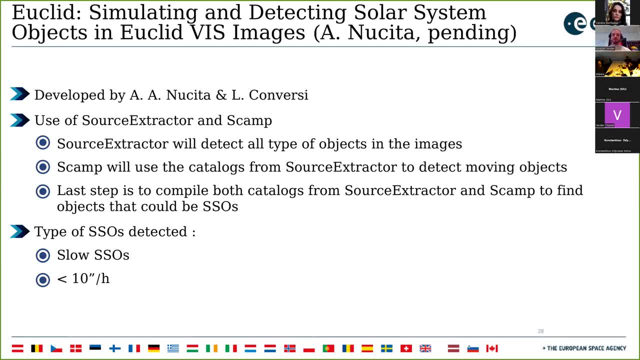 But we focus on slow SSOs, So it's a bit. It's another challenge And it is doable with Source Extractor, because then it will be small objects With very long streaks. Source Extractor is not very, very strong. 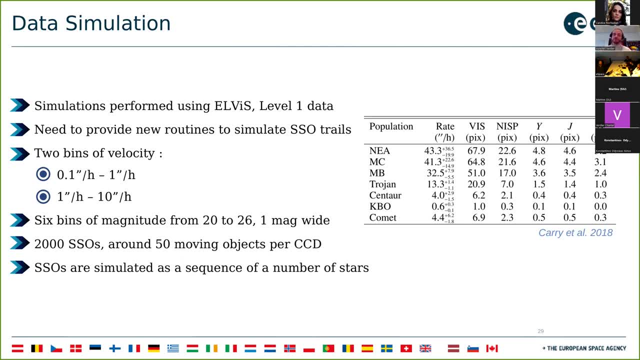 I wanted to talk about a bit the simulation we had to do because, of course, you're still not out in space, So we need to have simulations of what Euclid will see. So you have a lot of teams working on this: how a galaxy will look like, how stars will look like. 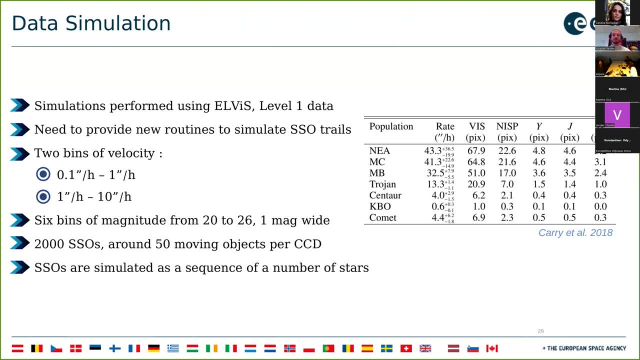 The problem is that the team doing that had never the time to simulate SSOs for us, So we had to do it like a homemade. It was before I came, so again, I did not really work on that, But I think it's important to understand that for now. 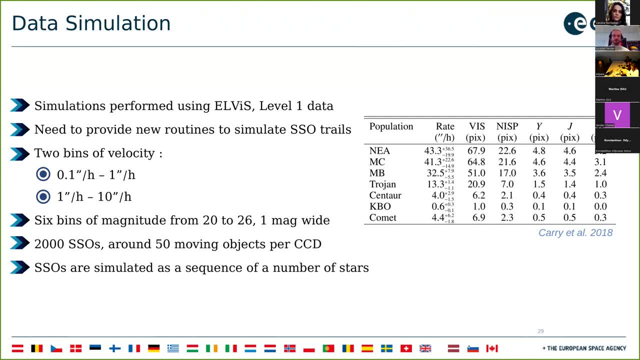 the SSOs we are working on are very basic simulations, So maybe we'll be lucky and we will have proper simulation just before the launch to be sure everything is working. It's a bit of a mystery because there is a lot of stuff to do. 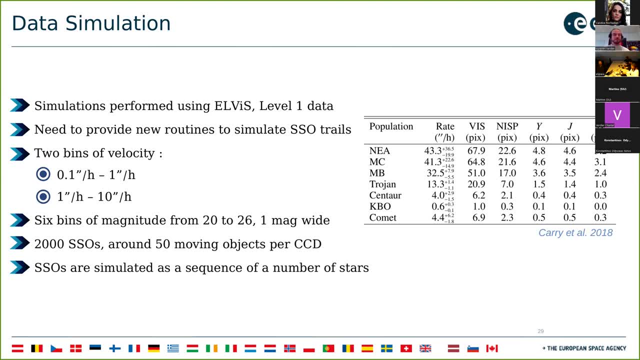 And now that the launch date is very close, I'm not sure we'll be able to have the information we need. But we have two categories of velocities, We have six categories of magnitude And so in one dither we have around 2000 SSOs. 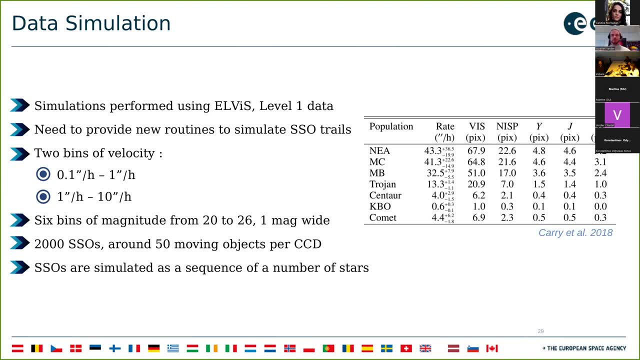 And we need them to work with that. Just to tell you, the SSOs are just to be simulated, just like stars just being put together And putting aside, and then they do a small tray and this is an SSO. So this is how it looks like. 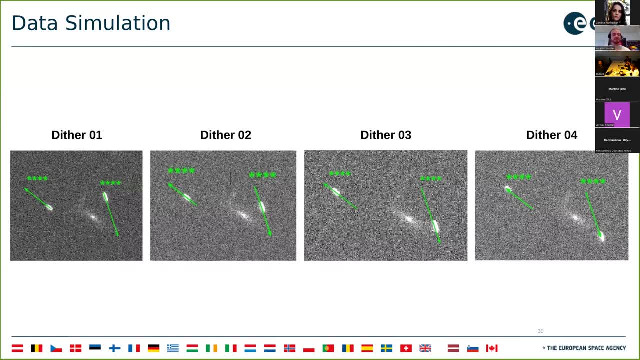 In this image. so you have the four dithers, You have the galaxy in the middle, one galaxy, And on the left and on the right you can see a small SSO just going around following the green arrow, which is what we simulate it. 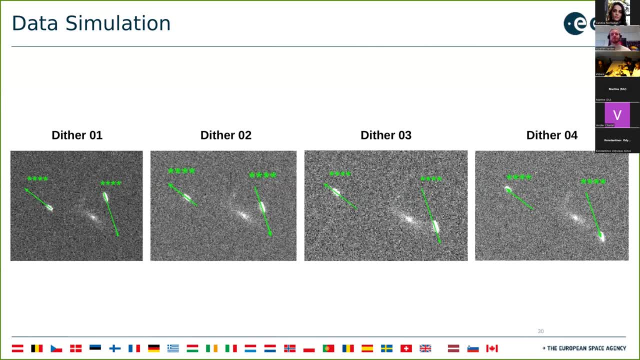 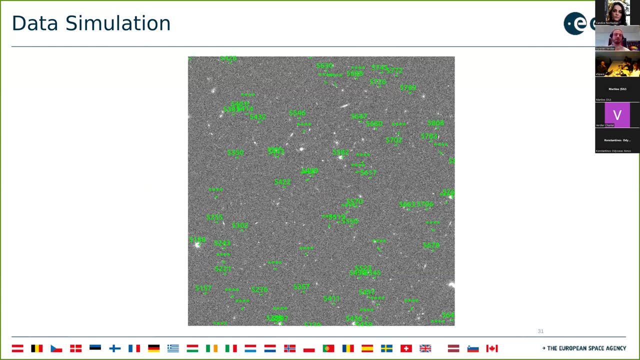 So now what we want is to detect this object in each dither And, at the end, understand that this is a moving object corresponding to an SSO, And to give you a more general visualization of one CCD. this is what it looks like with random SSOs in one CCD. 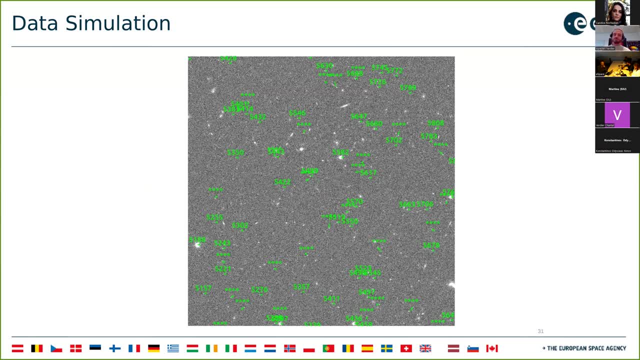 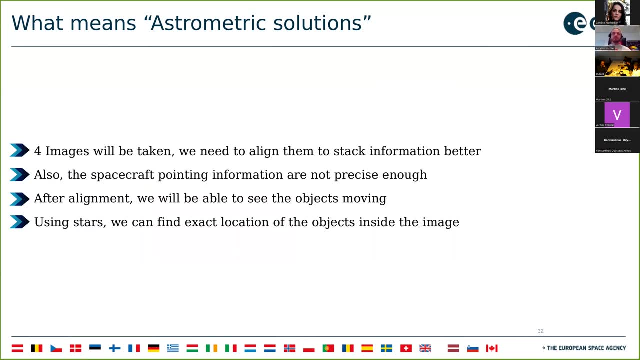 So there is still a lot of object to detect. So I was talking about SCAMP in an alignment and what we call is finding the astrometric solutions. What is this? As I showed before, Euclid will take four images that won't be perfectly aligned. 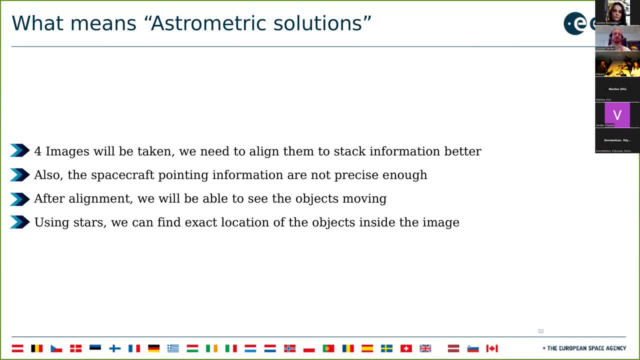 because they will be shifted to fill the gaps. So we will have four images that are not aligned. So we need first to align them. But even if we align them, the spacecraft is not very precise. We will know that he's somewhere, looking somewhere over there. 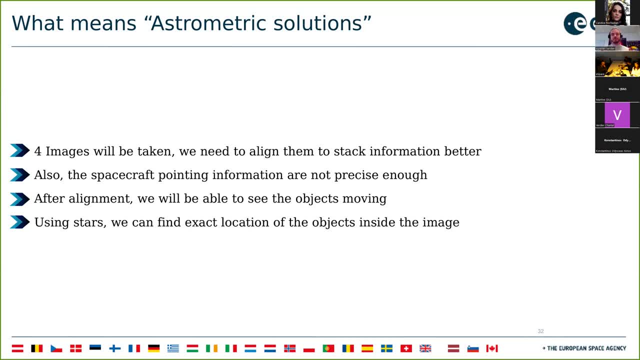 but not precisely where, And as we want to detect SSOs with a very precise, very precisely, we need to know exactly the coordinates in the picture. So what we do is we use the stars that are present in the image and we compare those stars with stars we know. 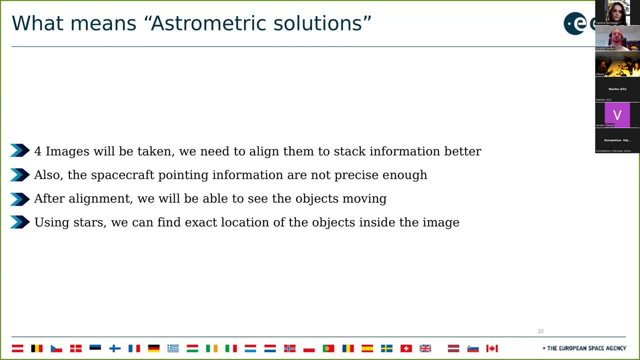 and we have the precise position of these stars, And then this is how we use the information: to what are the coordinates of each object in the image from the stars we already know. So this is finding astrometric solutions And you will see, it's important because it's had been mainly my work. 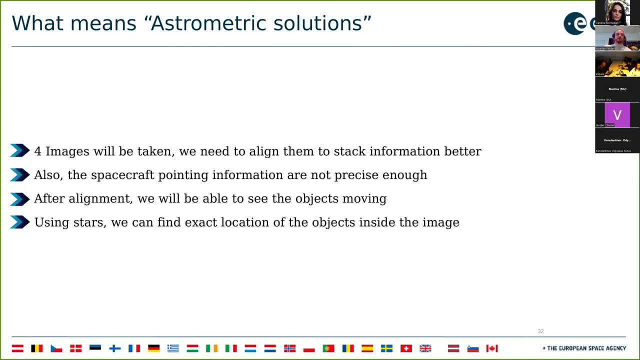 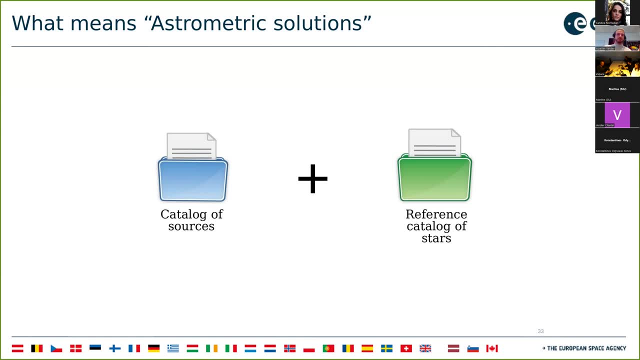 for the last month is to find a software that can do that precisely. So, as I said, you have a catalog of sources from your software that found all the object in your image. You have the reference catalog of stars. Here we use mainly Gaia stars. 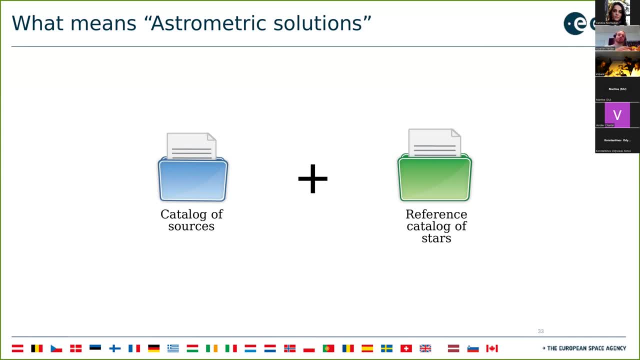 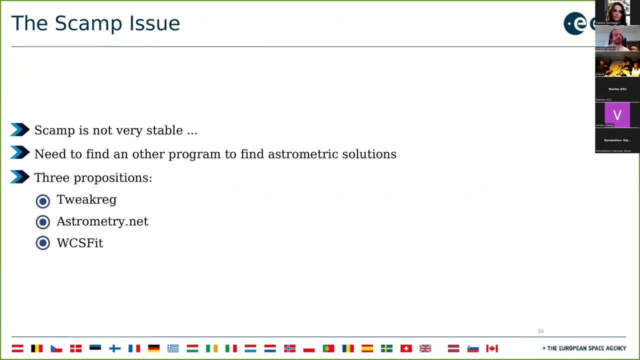 And then we see in the catalog of sources if we have objects that could correspond to these stars, and then we just align everything and we have the what we call the WCS information And then we have the information of the image. So SCAMP. 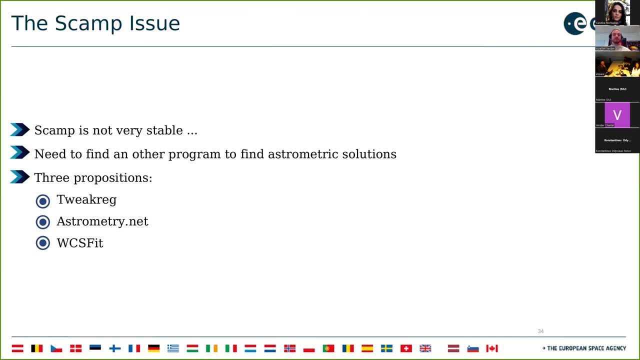 When I arrived, I had to work with SCAMP to check if everything is working or not, And the answer was, well no, SCAMP is not stable at all. Sometimes we had a problem with memory, So SCAMP is not very good with a huge amount of data. 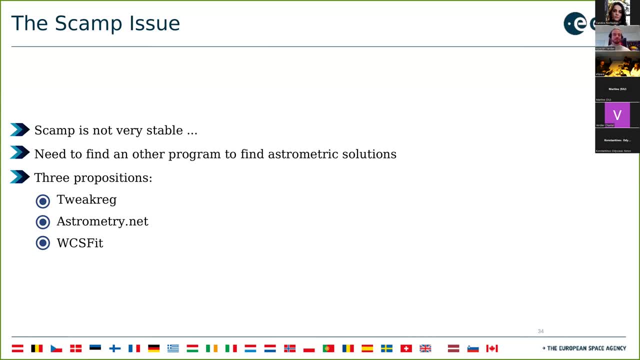 So sometimes we could just have segmentation fault coming from the program, just because he was not able to work with this amount of data, And sometimes it was completely random. We don't know why. We maybe just copy a file and with this file it's not working. 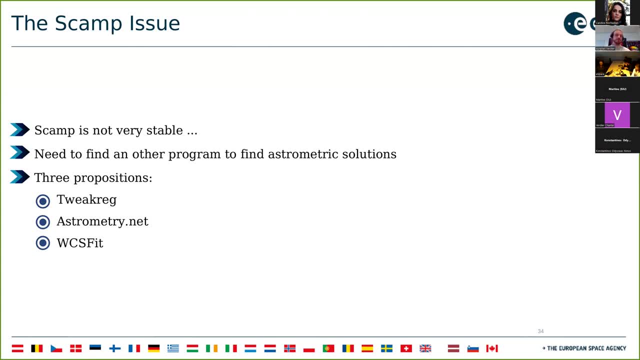 Sometimes the data was not very huge, but SCAMP was not working either, And we cannot allow ourselves to work with a software that is not consistent, especially for a space mission that will work for six years automatically, And so suddenly we have the data that are not available because SCAMP was not working. 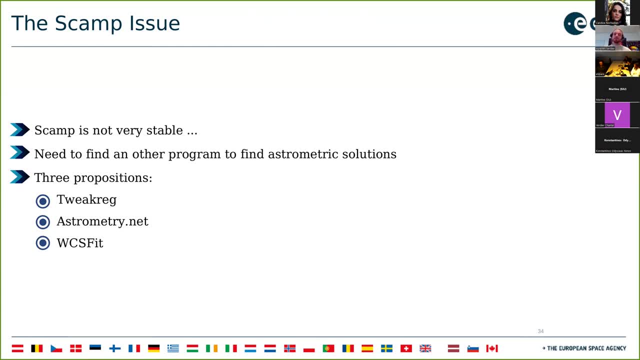 This is not what we want. So my part of my job was to find another way to do the astrometry solutions, So three propositions came. Tweakreg, which is the software used in Hubble, so it proved that it could work. 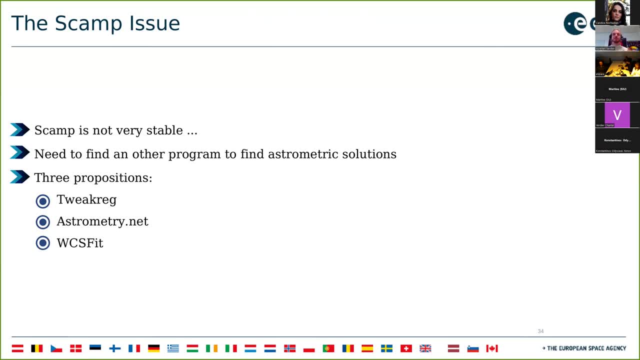 Astrometrynet, which is a software that is starting to be used in Euclid Consortium And WCS Fit With Tweakreg. I was working with someone on Hubble, but right now he's a bit buzzy, So the project with Tweakreg is on a break. 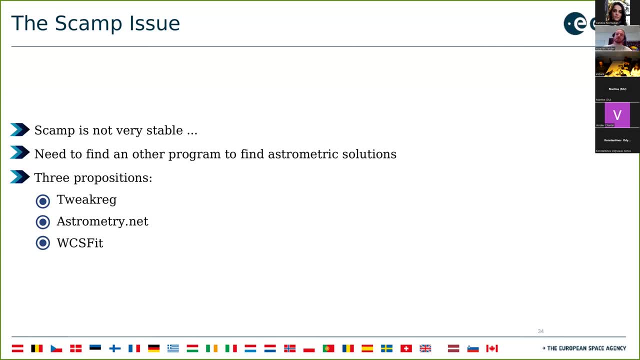 We had no time to improve it, but I had a lot of time to work with Astrometrynet And it was kind of funny and I wanted to talk a bit more about this one because all the things we have to think about how this kind of software works and how to develop. 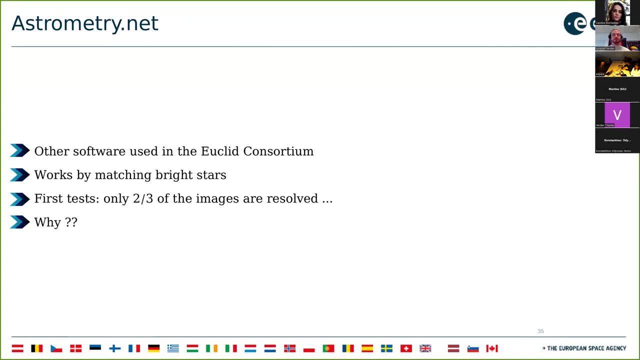 the pipeline around. it was very interesting. a bit frustrating too, And so this is why I want to insist a bit on this one. so basically, this one would just work with bright stars. so you'll try to find bright stars in your image. you find bright stars in the reference catalog you're using and then just try to match. 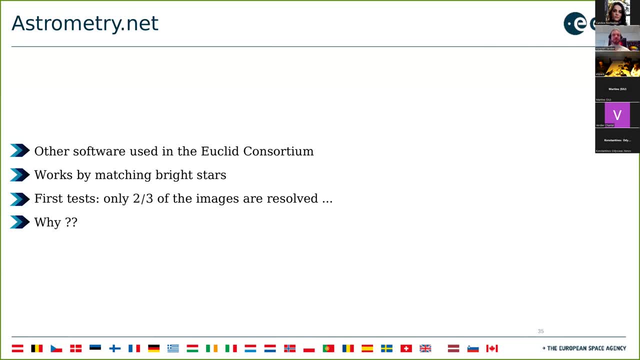 them. so when we were using our images, then we have only two-thirds that were correctly aligned- at least the solution was found- and the other one-third no solution at all. and the question is now: why? what was i doing wrong to to with this software? it should work like if it works. 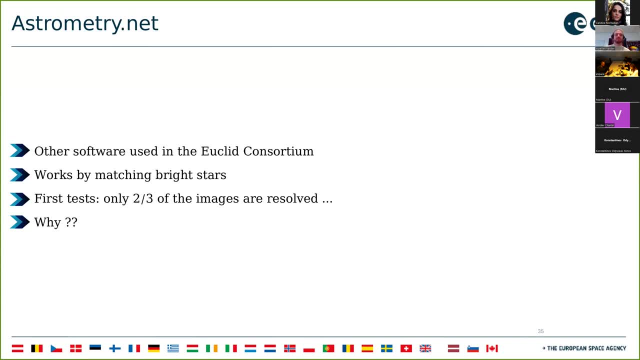 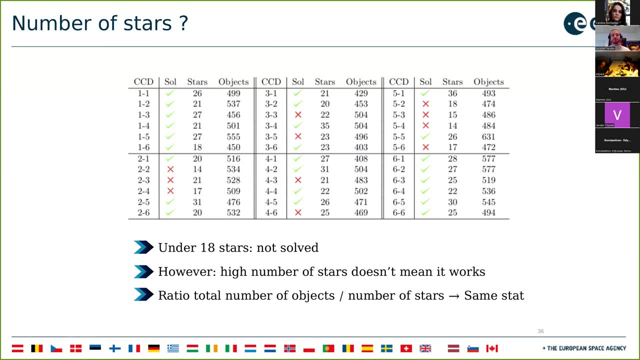 with one image. it should work with all other images. so what is the problem? well, the first question is number of star in one ccd. so i tried to count every stars in every ccds and the thing is that i was starting to see that under 18 stars it was not working. so i was like, oh, maybe this is. 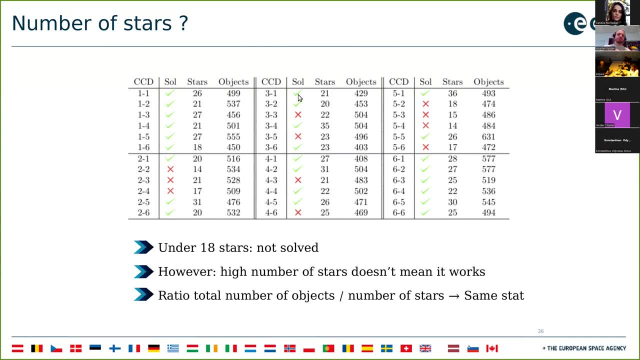 the solution. nice. but then suddenly i could find 22 stars, and it was not working. you or even 25 here, it was not working. so apparently the number of stars is not the problem, so maybe it's the number of objects inside the, the image and same thing. it was kind of random. 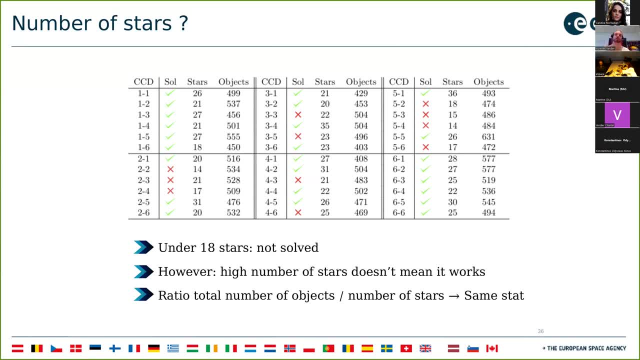 so then i started to think maybe it's the where between the number of objects and the number of stars. so again i tried and i had the same statistic as counting the number of stars. so nothing was changing. so let's try to find another solution if it's not the. 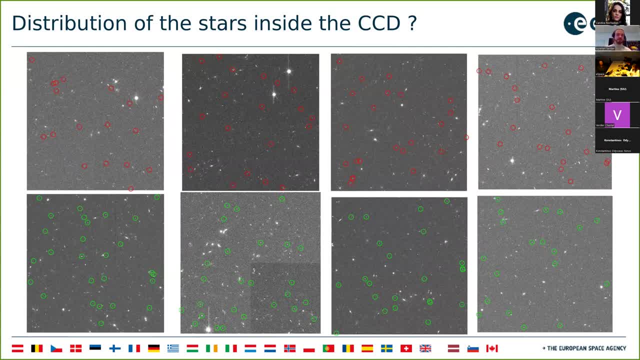 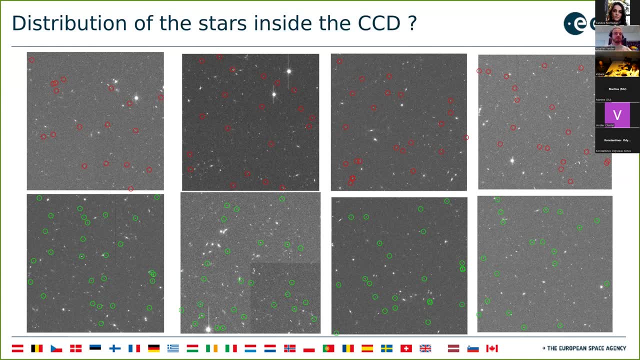 number of stars, maybe it's the distribution of stars. so then i tried to analyze where were all the stars inside the images and try to compare in between working images and not working images. here on top the red means that it was not working and on the green it was working. 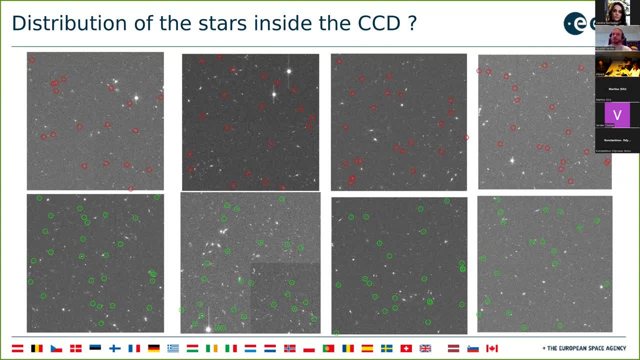 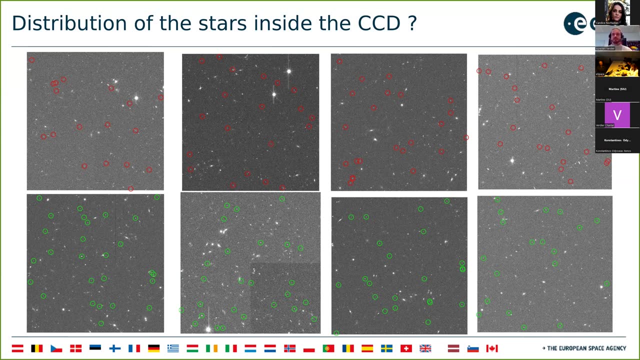 and by just watching all pictures i could see nothing really like, for example, a big hole or something like this explaining that it was not working the distribution way kind of kind of random and kind of the same for every picture. so it was not the distribution of the star inside the ccd that 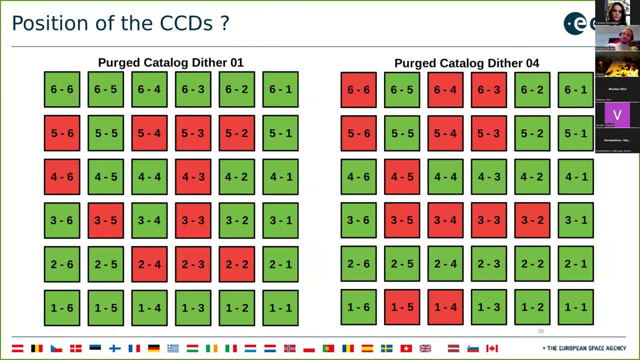 was the problem. okay, so now, what is the problem? maybe the position of the ccds themselves. so this is this, represent the whole image. the 36 ccds, the red ones are the not working ccds, and maybe you know if it was on the top, top left, on the top right or in the middle, only on the borders. 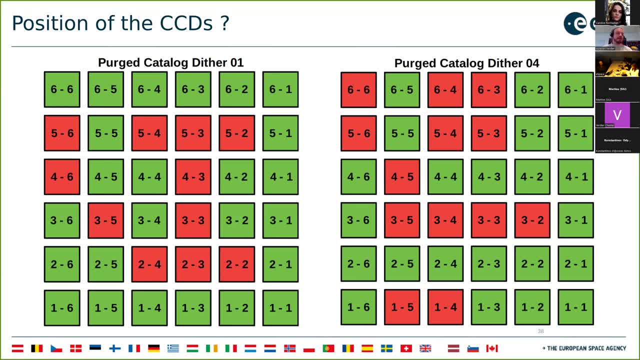 something. maybe that could appears everywhere and the answer no. it was kind of random. and the left, you can see you have a lot of stars and the red ones are the not working ccds and the red ones are on the some, some ccds not working in the middle, on the left and for the other image you have. 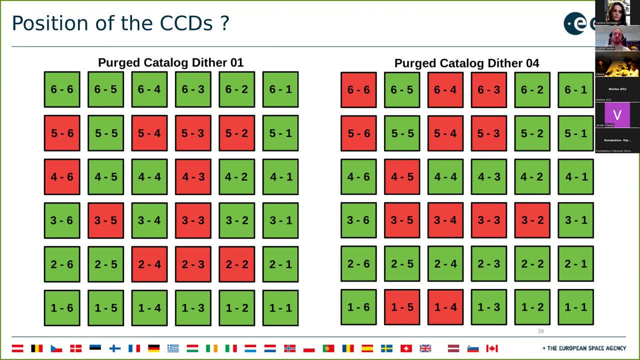 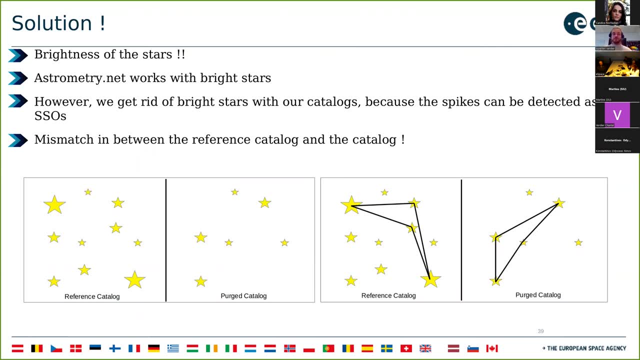 on the top left, also not working ccds, but also on the bottom. so again, it was kind of random, so no explanation at all. so what was the issue? well, i finally found it's the brightness of the stars. so, as i said, astrometry is working with bright stars, and what we forgot is that in our catalog. 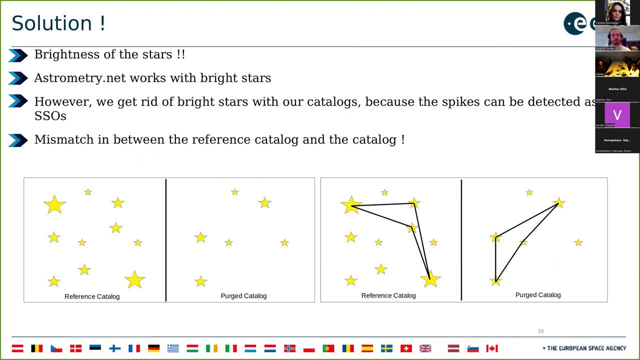 we used what we use, we what we call purge catalog, which means that the stars are not working, but the bright stars, the very, very bright stars inside an image have some uh, some faint. you know, like when you picture with too much uh, too much light, you have those uh spikes coming out of the 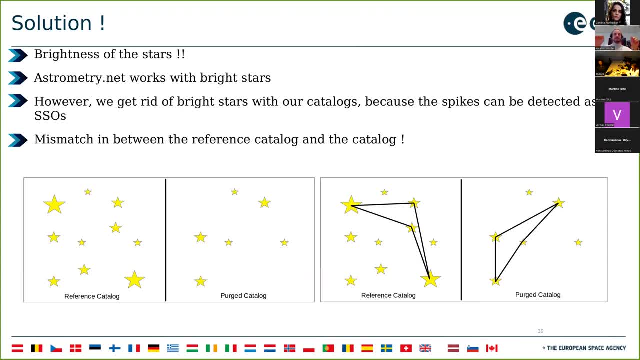 light. well, you have the same with euclid and so those spikes can be taken as uh ssos in our pipeline. so we just get rid of those stars and the spikes around the stars. so our catalog is missing bright stars. so why is it a mismatch? well, on the bottom you can see on the 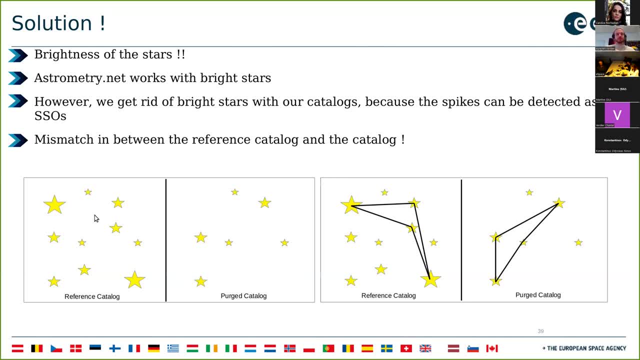 reference catalog you have this, all those stars, and on the purge catalog you have a few bright stars missing. so astrometry will go inside the reference catalog. he will take four very bright stars, because this is how it works, and create a quad with it. so then this, this kind of shapes. 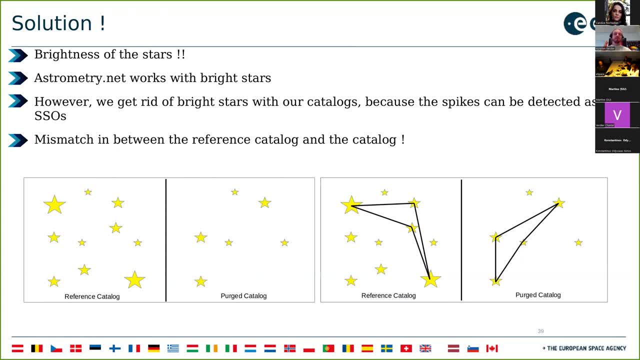 and he will say: okay, i have this quad and i want to find the same quad in the catalog i have. so when he goes to the other catalog, well, the problem is we don't have those bright stars. so we take all the bright stars and make another quad and of course, have a mismatch. so in the pictures where 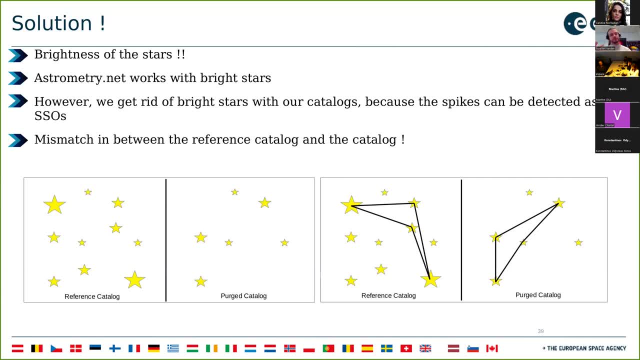 we had too much bright stars, it could not be possible for astrometry to work. so what we do is that we don't use the purge catalog we use, we use the full catalog, and then it was working 100 of the time. well, kind of 99.9 percent of the time. so way better. so now let's develop a pipeline. 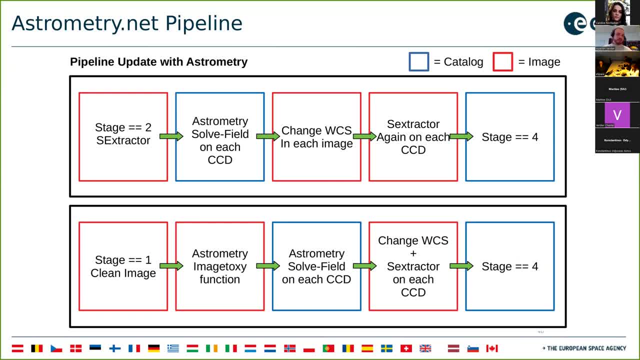 around astrometry. so i had two ids. the bottom one was not working because, uh, the, the function image to xy that you can see here, was not working with uh, with our images, so we had to cancel it. but the top one, um, we start from from a source extracted images, so we have the catalog of the source sources. 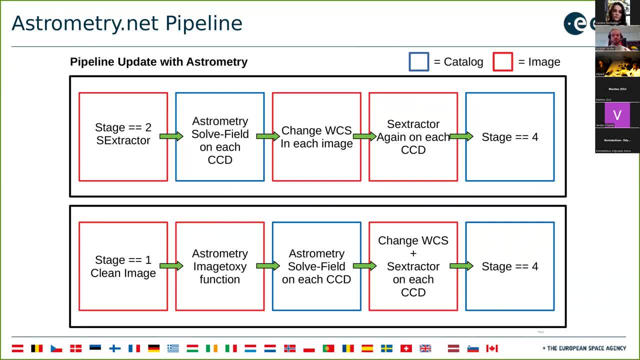 inside the image, then we use astrometry to try to to align them, using Gaia stars. then we change the wcs in the images to have the image properly aligned, and then we use extractor again, but this time to exactly find ssos. and then we can go on on the pipeline. so what did? but the problem is the. 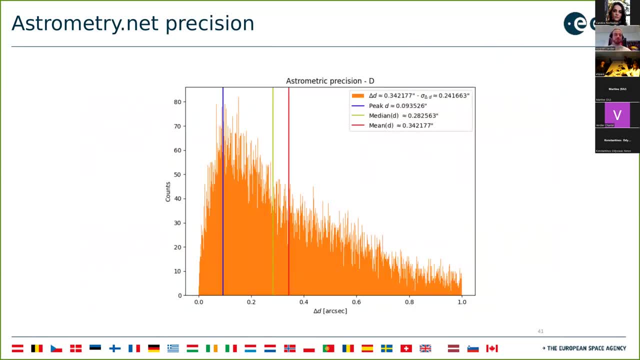 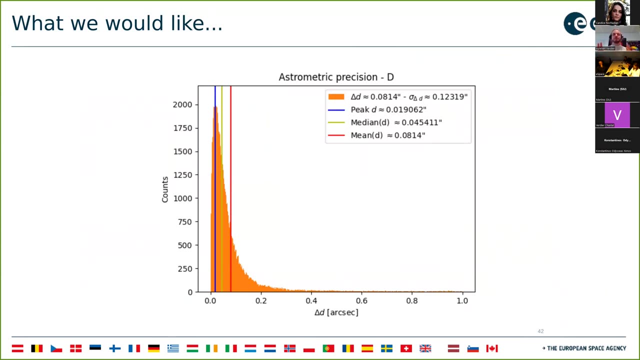 result was not insane. so this is a way to um to check if the alignment alignment is well done or not. so what we should have normally on very clean image is a beautiful pick and not very wide, and we want something close to 0.03 oxygens, which means that an object is 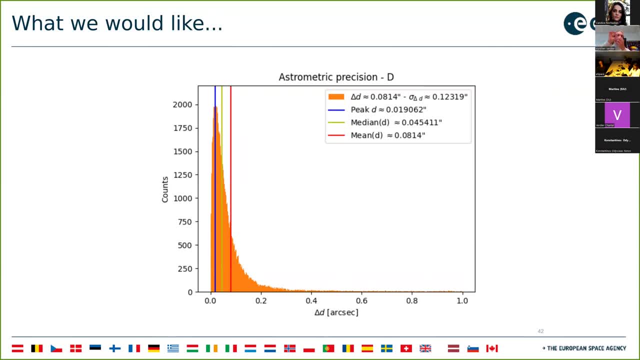 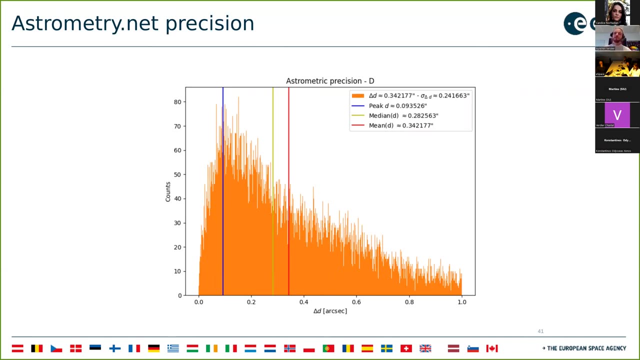 not further away from 0.03 oxygen from other objects when you align the images. so the same object is kind of the same position in the four images. uh, problem here is that first, the precision is around 0.1, which is not good at all for Euclid, and also it's very wide, as you can see, there is 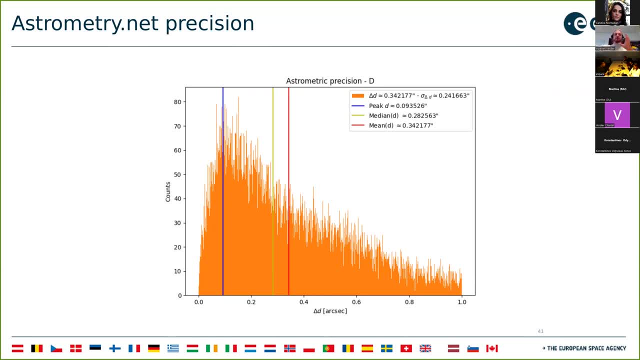 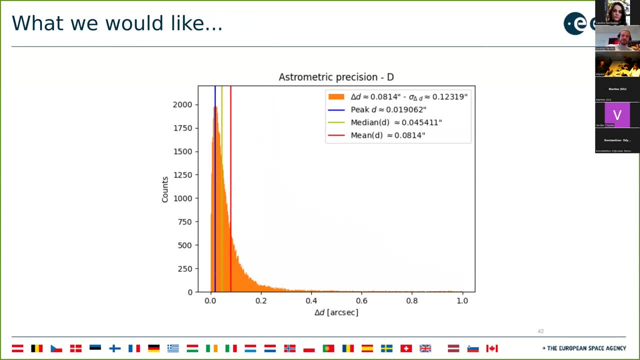 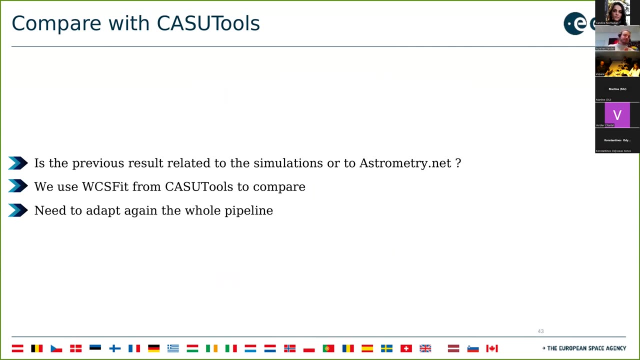 objects that are very, very far away from the other position in all the images. so it's not working at all. well, it's working, but not good enough. so why? maybe it's the simulations or maybe it's astrometry the problem. so now we go to wcs, fit and 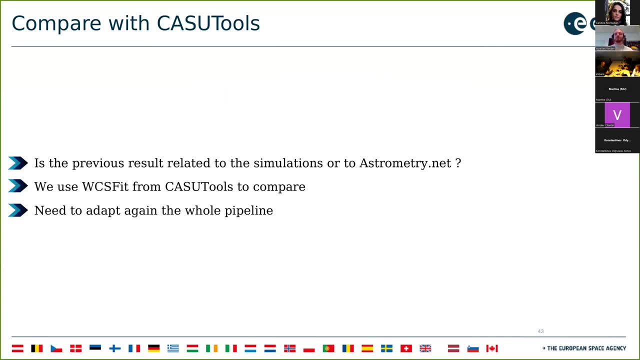 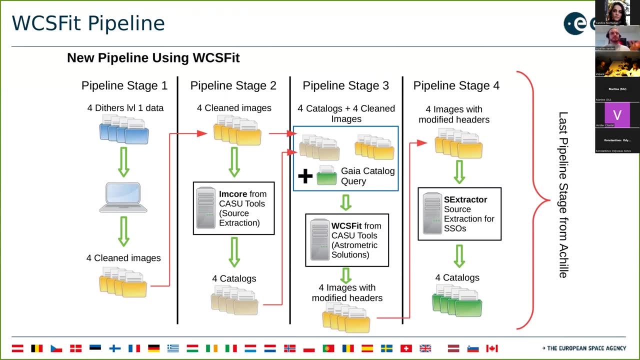 do the same job. we use wcs fit to try to align images and we see what are the results. so here is the whole pipeline for wcs fit. so the first stage is: clean the data. okay, this is done. then pipeline stage two: we use this images and we try to find sources using a source extraction software. this time we don't use source. 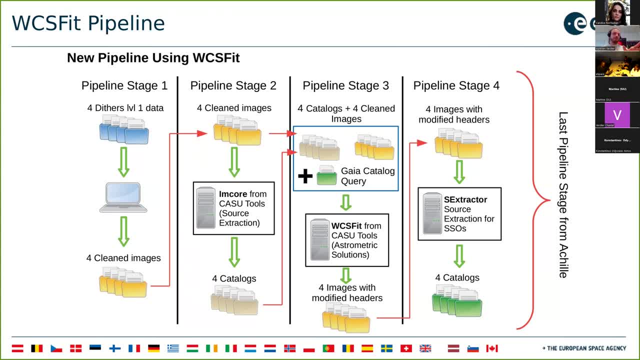 extractor because wcs fit needs i'm core, a type of file, so this software to have the catalog. so we use i'm core. we have four catalogs. we use those four catalogs with the stars and we send it to wcs fit and then we try to align the images. then wcs does the work, change the of the images and we 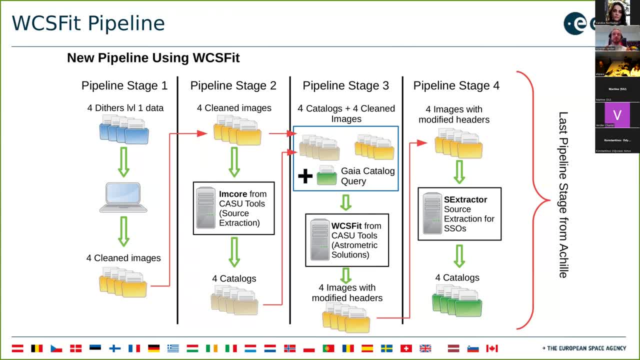 get four aligned images, then we use source extractor on those four images to then try to detect objects, including ssos, and then at the end we have one last pipeline stage to only find ssos precisely. well, here are the results. it's way better wcs fits can work with this kind of data. 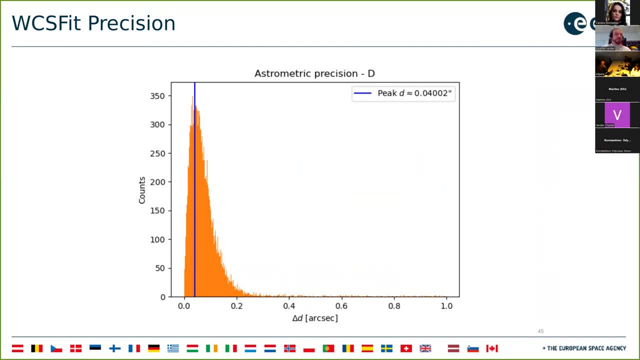 so it means that astrometrynet was kind of the problem. um, so we just took the decisions two or three weeks ago to use wcs fits instead of astrometrynet, and now the pipeline is completely ready and we just have to do more tests with new simulations. 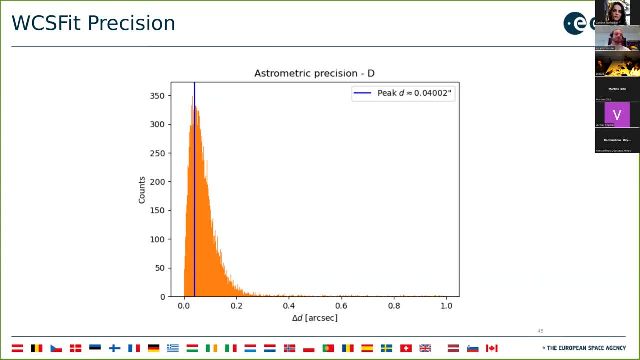 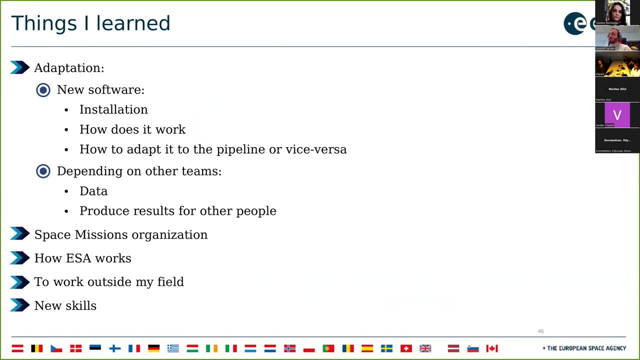 if they come, and they can just use it when the Euclid will be sent. so it's kind of nice- nice too for me to finish on a good point- having a proper pipeline working and not something kind of messy with astrometrynet. um, so yeah, I've been working on this for 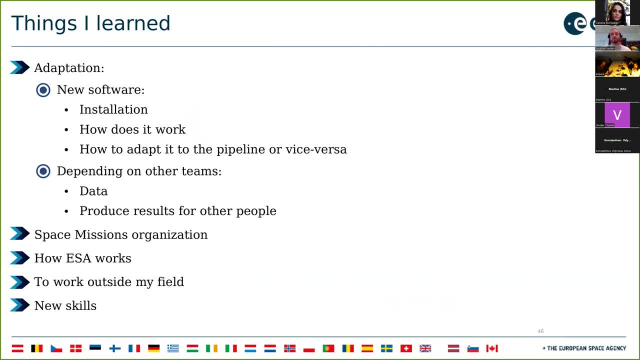 two years, uh, and I wanted to talk about what I've learned from Issa and from my work. so first thing is adaptation. uh, I've only knew the source extractor software before I came here, like in all the software's. I've been working for two years here, and so I adapt to a lot of new, new software. 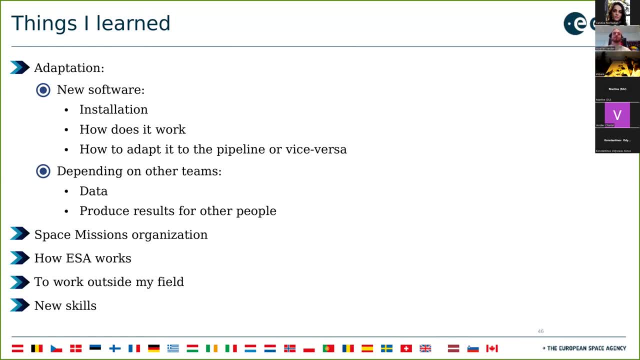 so how to install them, to have to understand how they work, how to adapt the pipeline to the software's or to adapt the software's of the pipeline, uh. so it was kind of interesting, sometimes exciting, sometimes frustrating, but you know, it's uh, it's adaptation, uh, also on isa you. 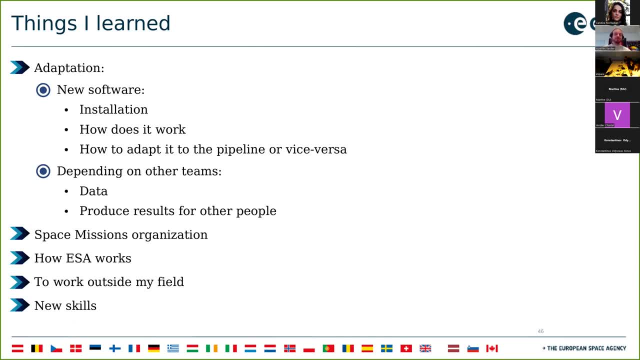 work as a team, so you you wait for data or you need to provide data to others, so you have to adapt your way of work to all the teams. uh, depending on you, and which you depend on too. it was my first work outside academic and in a space mission organization like a big one. 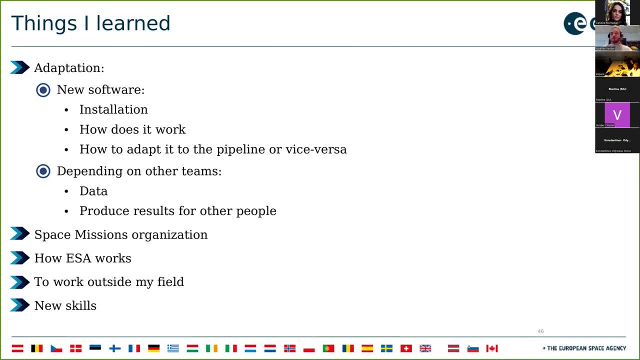 which is isa. so i learned a lot about how a special mission is organized. and yeah, it's. it's kind of interesting to know when you were inside, what are the decision taken. sometimes you're kind of surprised, so it was very interesting to know what was going on. 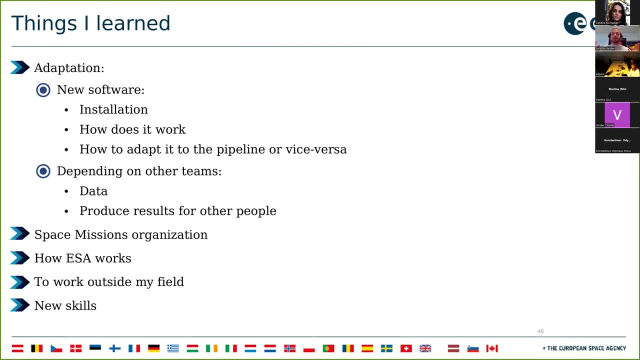 and also how isa is working, because from my point of view, from a very, i would say, naive point of view- issa was a lot of scientists being all together very happy to do science, but it's not administrative and how to handle teams working then on the science. so it was very good for me to 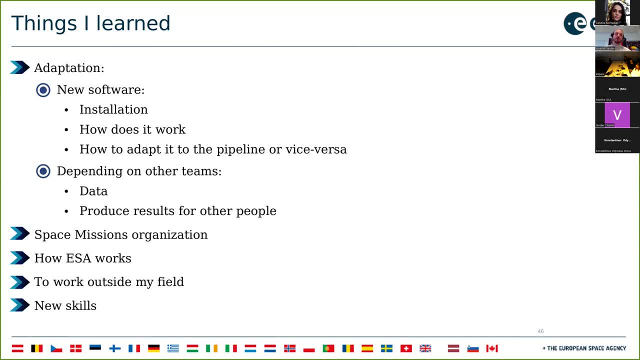 understand how issa was working and then how i, how i could help this and where i want to be in this big chain of space science. uh, also, i was a bit working outside my field. normally i'm more into dark matter, dark energy. this is why i like euclid. but then i was going to work on planetary science. 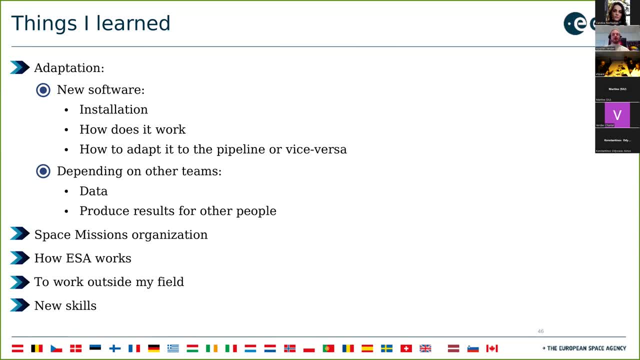 so it was very nice also to just go a bit of the field. i like, uh, to discover new things and how it works in other fields, so very interesting too. and finally, of course, from all the new softwares and everything i had to do, i have now new skills that i think will be very helpful for later, for 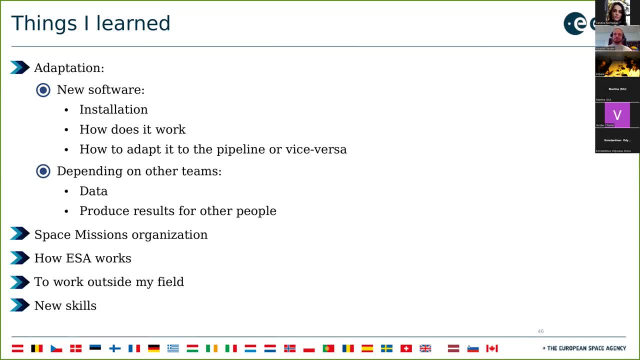 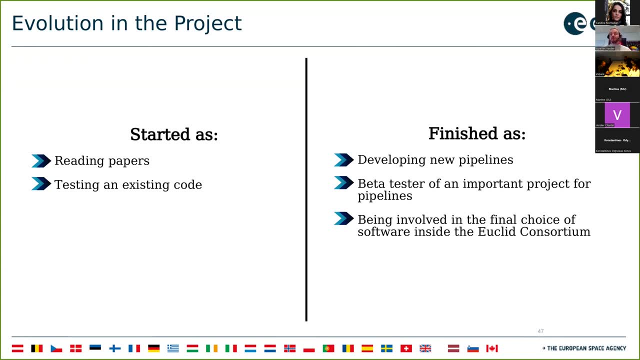 the next, next, uh, the future of my profession, also my personal evolution in the project. so i started as uh, you know, with the co-op and stuff, just reading papers, testing code. everything was going a bit slow, so it was, uh, it was interesting, but you know what like, okay, i'm just the new guy, the new young guy, just trying. 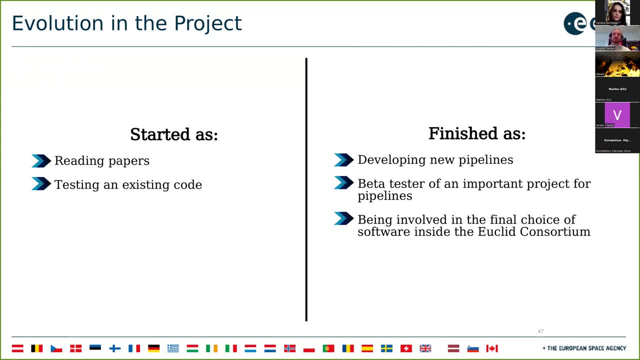 to do stuff, maybe what? what will happen after the two years? well, as i finished, i'm kind of very happy of the work i could do. i could develop new pipelines, just not test one, just develop new ones from from the the early ones. so very cool. now i'm kind of beta tester of an important project. 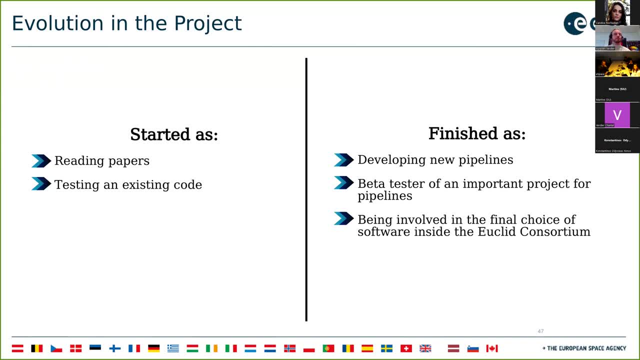 for pipelines which is called pipeman. that will be using whole isa for a lot of space missions. so i'm directly connected to this project and i'm doing tests on it and also in the euclid consortium. we still haven't chosen the program we want to use officially in the different pipelines. 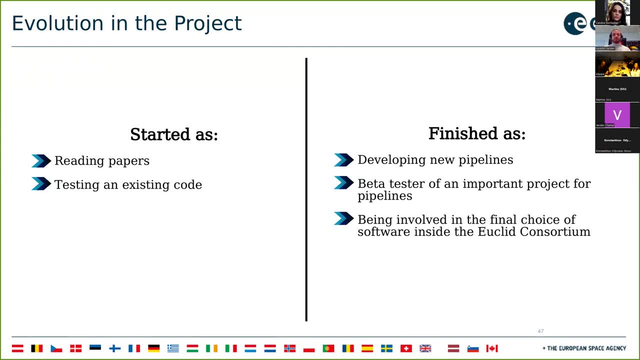 of the whole mission and so people are coming to talk with me about what i think, uh, of all the software i used, how we should use them, etc. so it's also nice to feel that now i'm part of the team and i can discuss with them and give advice or learn stuff, and i feel i'm a part of the the euclid team. so it's. 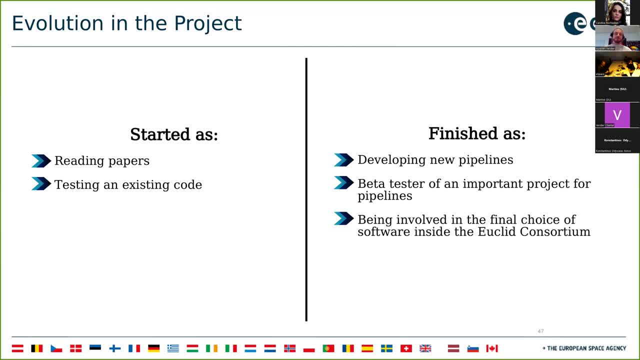 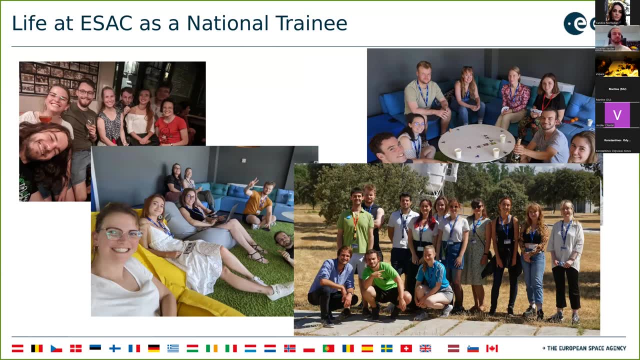 it's very nice to end like this: the, the internship. i've been talking a lot about work, work and work, but not only work. ygt's program is also about the, the, the new people. so i met a lot of amazing people, i would say, from other countries- canada, spain. 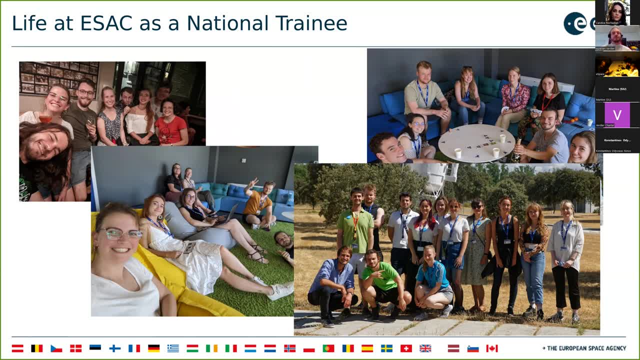 germany, sweden, france, etc, etc. it was very, very cool to meet all those people, to just have fun together, sometimes playing cards or going out in madrid. so also there are young people at issa and it is very interesting and very nice to meet them and be with them. 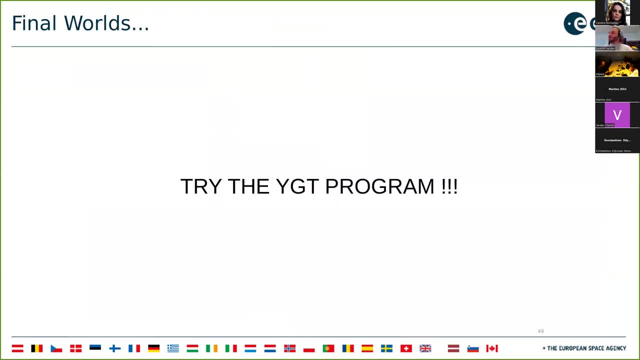 so what i would say the last words is the yg program. if you can, if you just finish your master, try to apply. you won't regret it. it's very nice and we need. if you're swiss, we need more swiss people in in issa. so please come and represent our beautiful country in a space mission, because 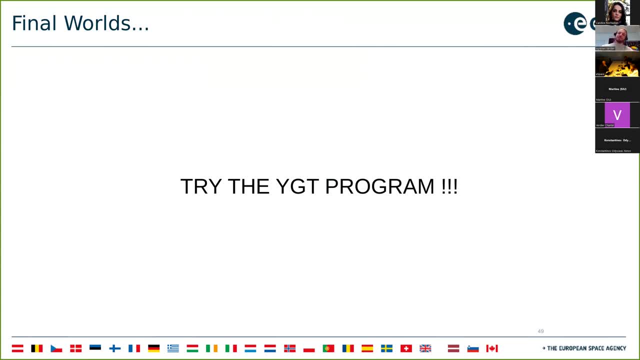 we are good and we need to show it. so thank you for intention. if you have any question, please ask us in the chat. thank you very much, um. so i think there was a question in the chat from belen and it was referring to slide 32, i think, um, and the question is: what's the time delay between the four exposures? 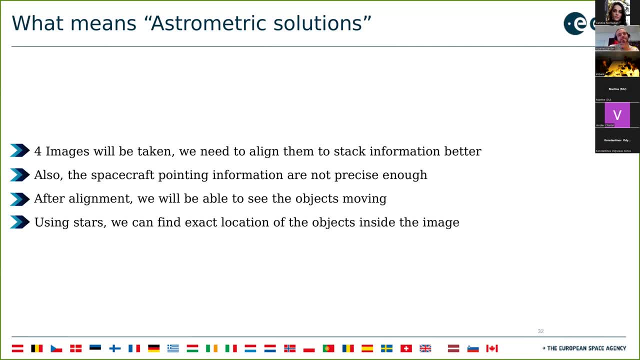 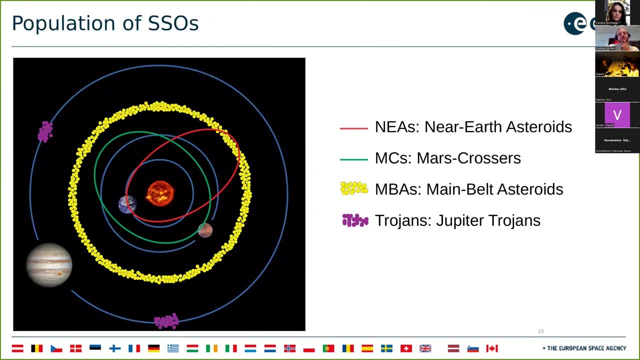 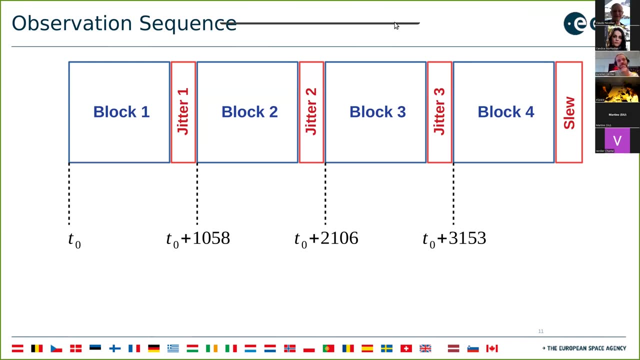 um, so between the four images, um, it's around ten seconds around. i think i showed it here. so in between each detail there is around one thousand seconds. okay, thank you, and i think claude has a question. i'll just, yeah, do you hear me? yes, okay, thank you very much, orellana, for a nice presentation. that was really. 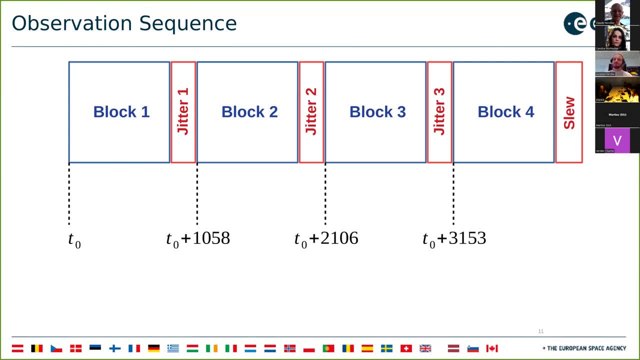 really good congratulations and also thank you for sharing your your thoughts about working at ESA. of course worked at ESA for quite a while. I didn't do too much administration and I was in a world where administration was very far away, but I guess it depends on which sector of ESA you work on. I have a question about the sky map that you. 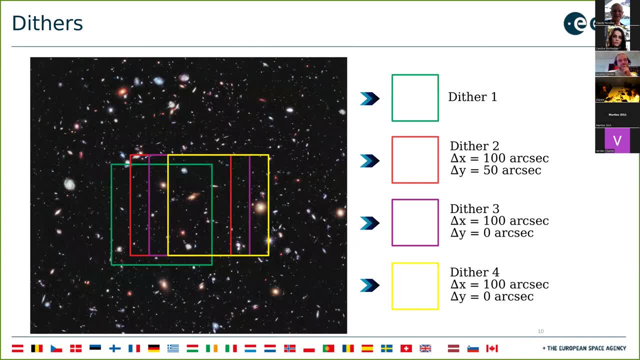 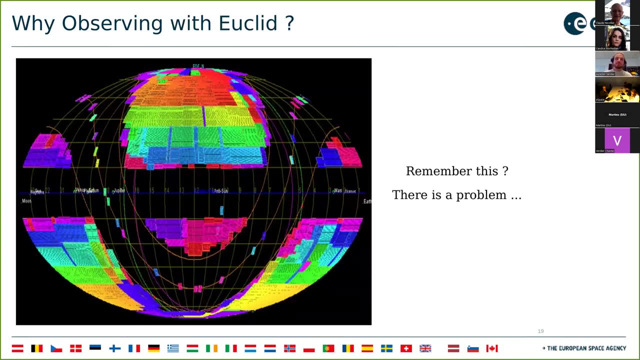 showed about what Euclid is observing, and these are the colored areas- and I guess this is a map- with the horizontal line in the middle being the ecliptic. is that right? Yes, And the other one is around the galactic equator. is that right? Exactly Okay. now I understand why there's exclusion around. 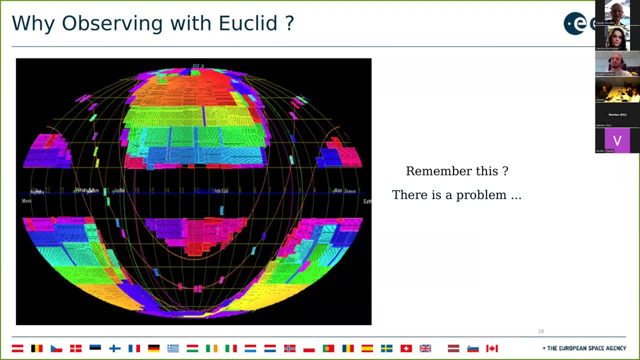 the galactic equator because you want to look at extra galactic objects, so you don't want to look through the dust and gas inside the plane of the galaxy. but why do we have this exclusion around the ecliptic, The eclipto along the zodiac in a way? why do you have that? 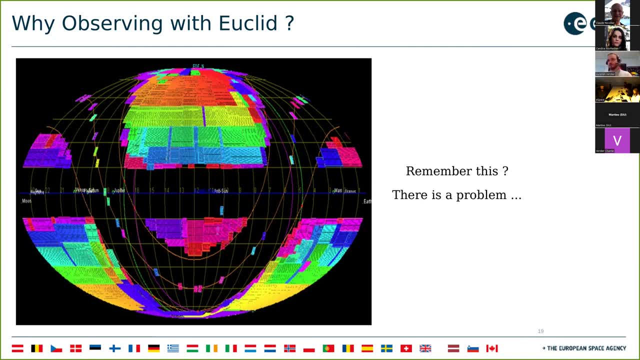 So first there is the sun that you want to avoid. Yeah, I understand, I understand. but except the direction of the sun, there's the whole rest of the area where you could observe. no, Yeah, so from what I've read, so it's been a while, but I think just that we really don't want any. 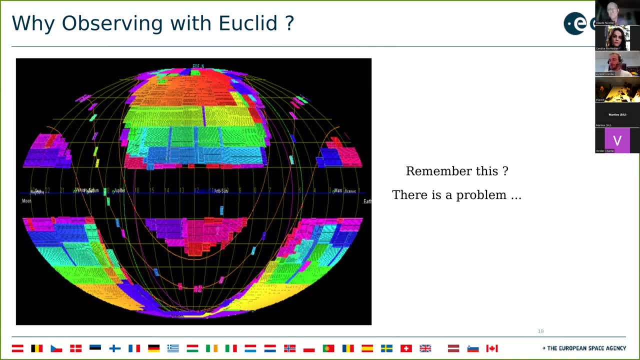 kind of, as we want to do, cosmology. you really don't want any artefacts inside your images. you want to have precisely what we should see outside our galaxy. so the problem is with those asterisks, with all the things you could have going inside the solar. 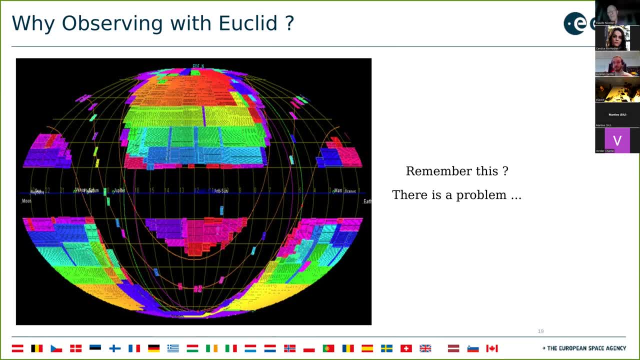 system it could create artefacts. that because we now detect SSOs. but at first Euclid mission was not about to do it, it was just looking at the sky and then directly work on these images. so we will help a bit detecting those artefacts with the solar system objects. 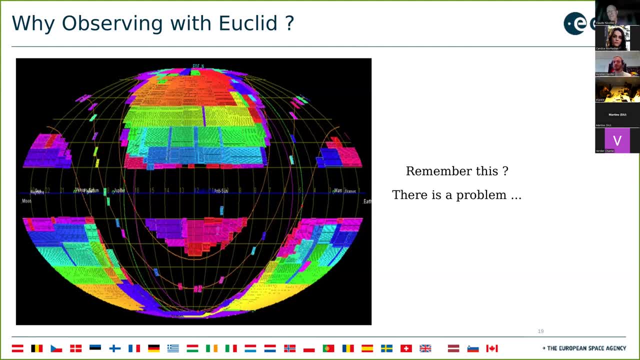 Euclid is not made for this. there is not a pipeline or anything else to just filter everything in our solar system. so we really want to avoid any artefact. to be sure we are looking at cosmologic objects. Okay, I understand. so they want to avoid artefacts because there would be an asteroid. 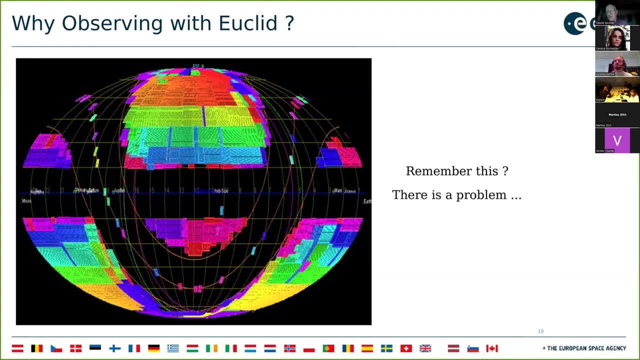 another object that would disturb the observation of objects in the extra galactic world, and of course we avoid also the plane of the galaxy, for not artefacts but just the dust and the gas. Okay, I understand, thank you. So in a way they block the region around. 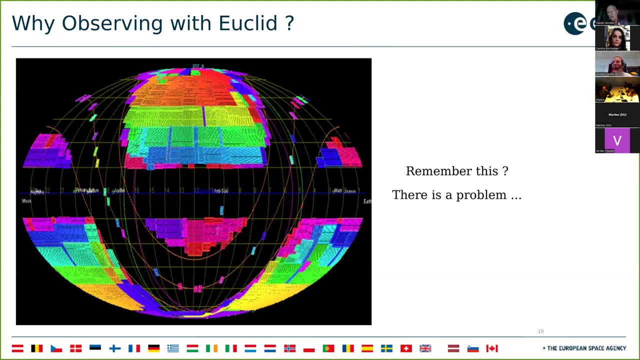 the ecliptic which you would like to have, but of course, your objective is not the primary objective. Yeah, exactly, we cannot ask them to change the whole mission for us. Okay, I understand. well, that's quite interesting. thank you very much. 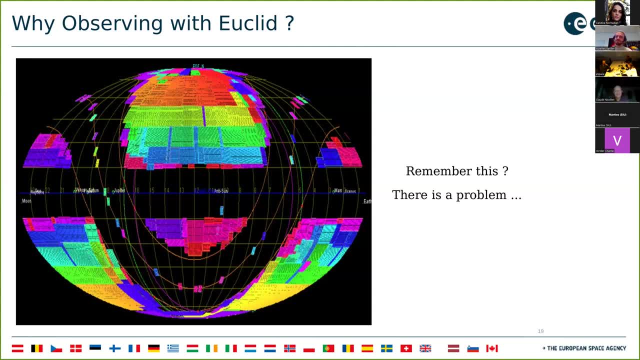 Thank you, And we have questions in the room here from Stefan, our colleagues. Yeah, thank you very much for the interesting talk. I have actually a few questions concerning the. at one point you said that you are going to also like interpret the data in terms of trying to 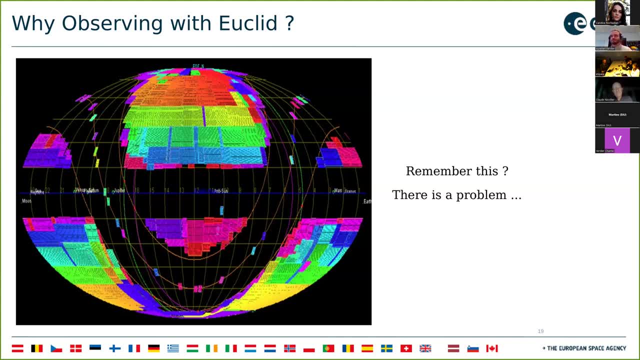 estimate rotation, property, rotation periods and other properties of the objects. so, but I mean this requires a lot of observations for each individual asteroids. Did you check how often you expect to observe each individual asteroid, or Are you trying to combine your data set with other available data sets? 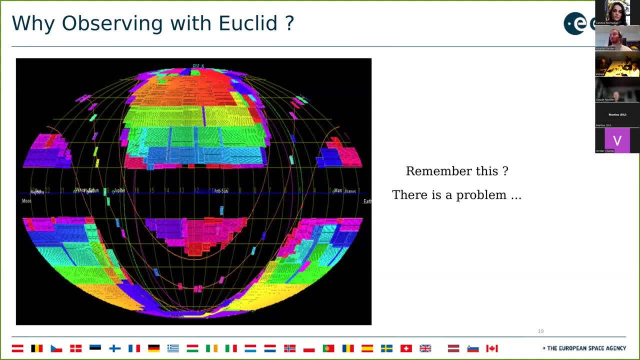 Yeah, so this is still on the work also, because we'll see, we'll say that the mission started like the, the ID to detect SSO started like five years ago, something like this, even more, And with what Euclid was proposing, with the hour-long observation of the sky. 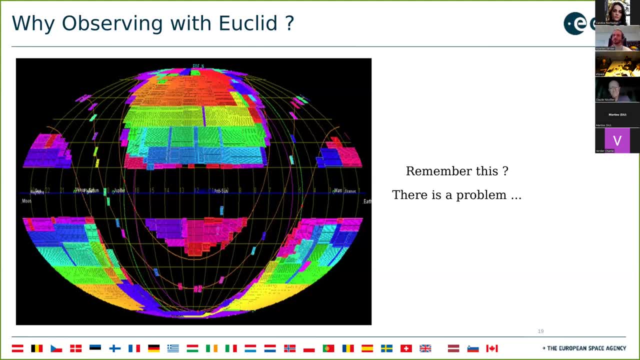 we would have a lot of information about the SSO we detect because it's very long observation time. So from those observation time and the very precise, like Euclid was very, very precise. so with the small amount of changes in light or anything, we'll give information about. 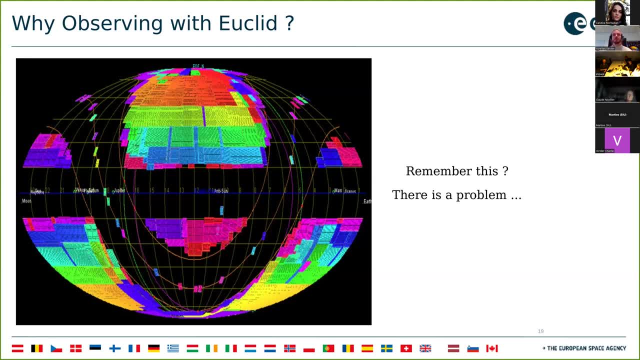 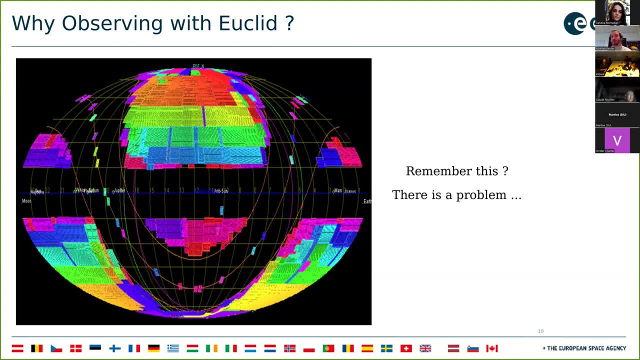 very, very much slower and stuff. We would be at this point right now if everything went well, trying to actually show that we can do it now. But, however, we'll have to do this in the next month and maybe wait for Euclid data to show that it was possible. So, because Euclid 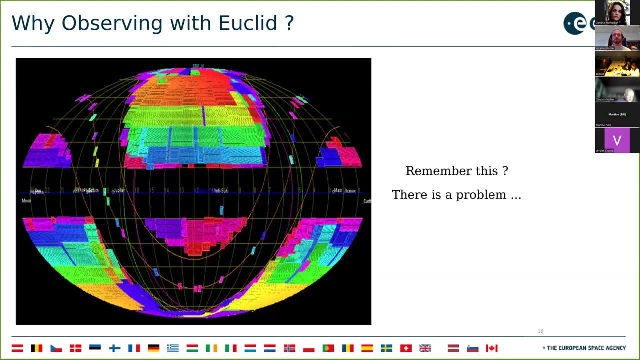 will be very precise. we think it's possible, But for now there is nothing done to actually detect this. Okay, so what? what's the exposure time of each individual images? It is one 1000, 13.7,, which is slice time, and one thousand 3 × Groene, performing an image for each innocent person by proximity: One hundred thousand to. 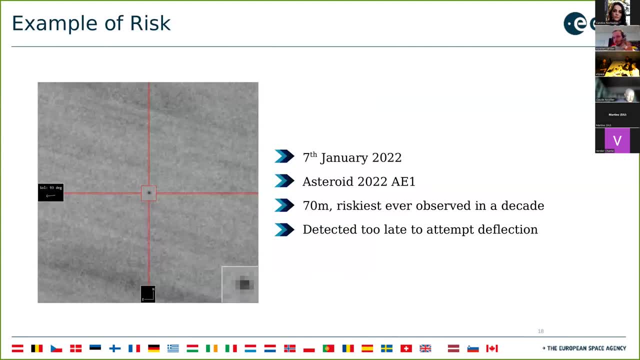 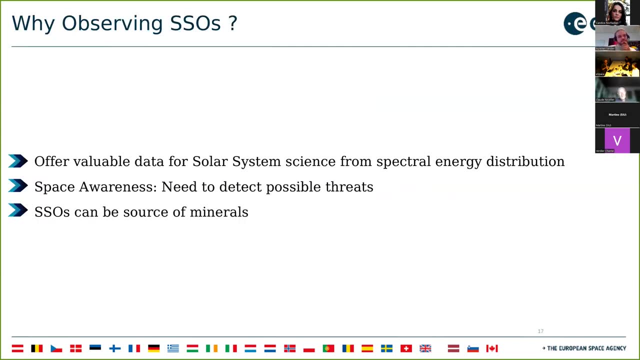 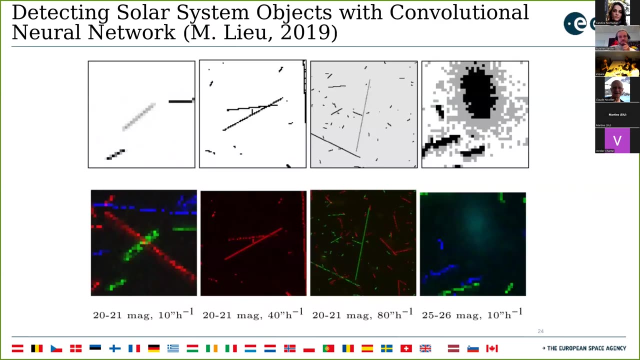 seconds, 1000 seconds. okay, around around. it's changed a bit every time, but it should be around 1000. okay, cool, thanks so, and concerning the plate solving, you said you were using astrometrynet in the first place, but you were not really um satisfied with the results by this. you changed. 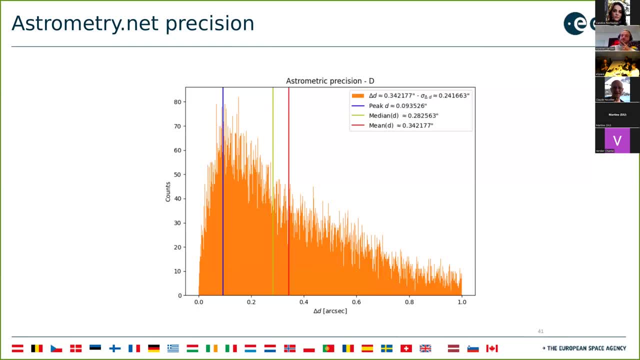 to. i don't know what other method wcs fits. yeah, so did you. do you know what kind of solution astrometrynet uh in the end used? so did you just use a linear uh solution for the whole frame or for each individual ccd and then maybe the, the other version, um, or the other method was? 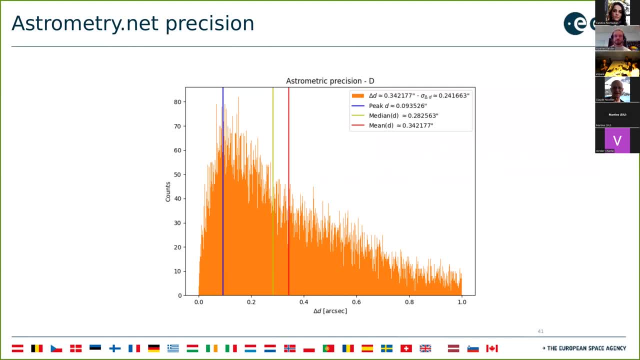 using a higher order uh solution so that this in the end, gets much more precise, or so, um, for astrometry, uh, what i know, because i've read a lot of papers because of this uh, is that, as i said, it's using quads build from bright stars. so what it does is that it trying to matches, uh, these quads. so i don't. 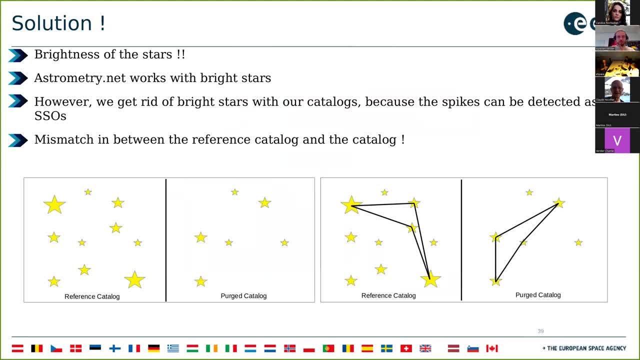 know if it's linear or exactly if it's linear or not. but i think the problem is as- uh, it's very bright stars- you don't have the exact center of the star. you know it's very bright and very large, so maybe astrometry will take the center of the star a bit here or a bit here, so the quads will. 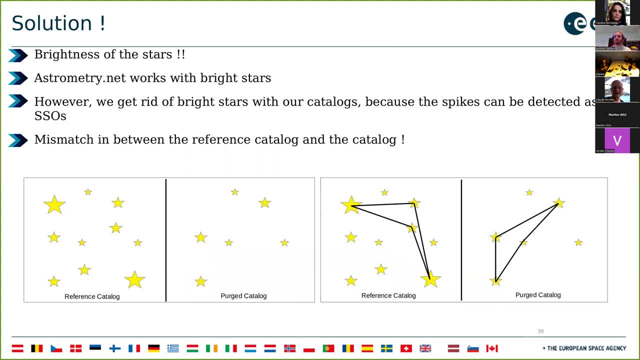 be a bit moving, depending of the brightness of the star and the center of the star and the center of stars, and so this is why it's not precise enough at the end. so one test we wanted to do is to maybe don't use very bright stars, only the less bright stars, but then the problem is that you might not. 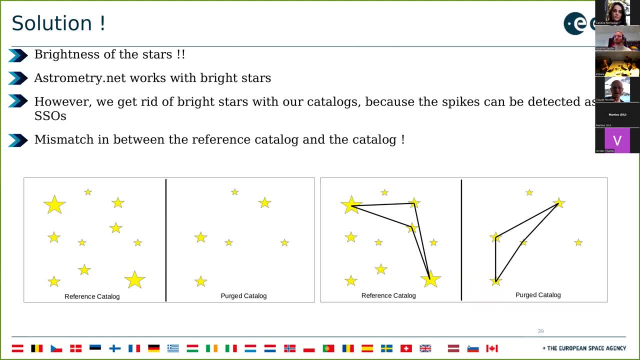 have enough stars and stuff, and even with this, this is how i managed to get, like, uh, 0.09 instead of 0.093. so even doing this, we still haven't a good solutions for this. so i think the problem is this is using the position, the exact position of bright stars, which is a problem because 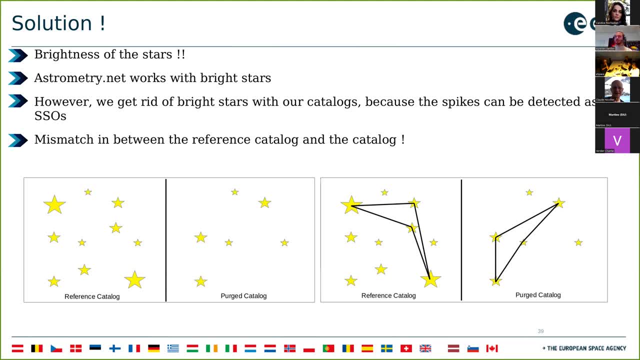 where do you put the center of the star at the beginning? yeah, okay, thank you. so. so maybe an idea would be to maybe, because, like, start with bright stars, because then it's easy to recognize the patterns, you don't have to correlate so many sources and then have an iterative approach and 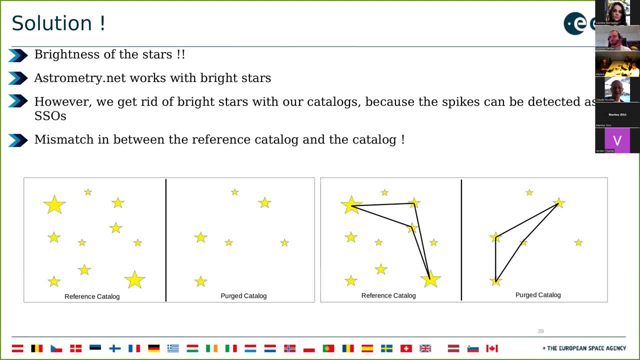 consider fainter and fainter stars, and then disregarding the, the bright ones, because the errors of the bright ones are, as you said, too big. yeah, that was one of the idea, um, but as i had the not good, not a huge amount of time and i wanted 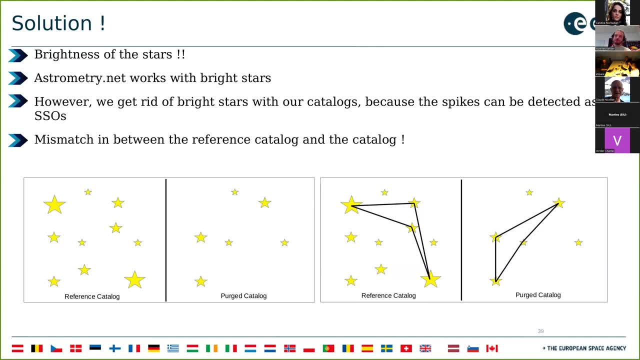 to be sure it was because of the itself and not the simulations. i tried wcs and it worked perfectly fine. so before i leave, i wanted to to do something working, so this is why i just went to wcs, fit, but yeah, the next month- like there is some people still working on this, uh, the next month they. 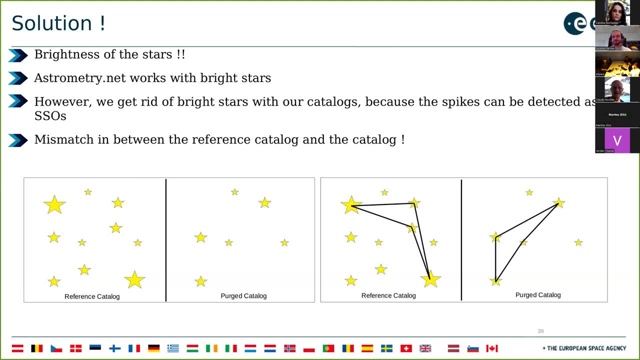 could do that, because this is still something we could do. yeah, and then final thing was: yeah, so you're, i mean you're, you're going to discover a lot of asteroids for euclid, i assume, uh, and these discoveries need follow-up, are you? are there already any plans for? 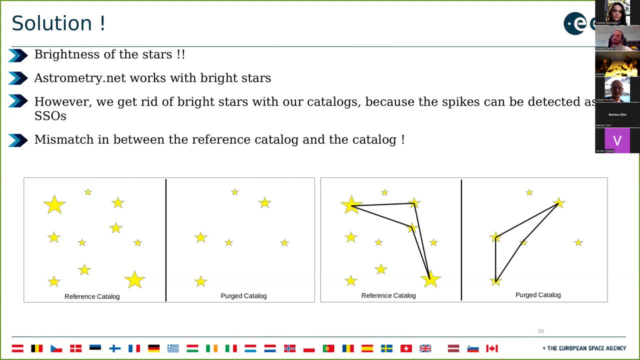 like a ground-based uh telescope network or are you working together with, like the optical ground station from ether, for example, to give the follow-ups, or are you? so there is a. there is a project called think uh. if i'm not mistaken, it's a project called think uh. it's a project called. 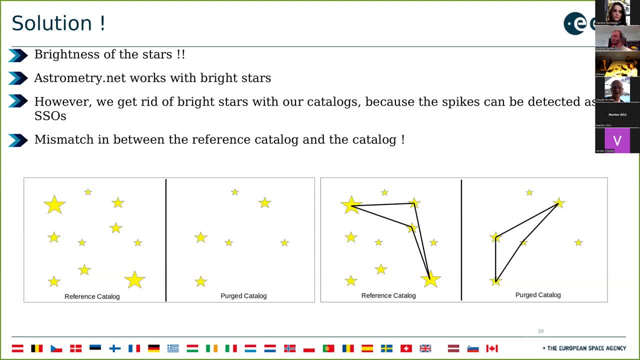 i n k, i think think of link every time i'm- i don't remember if there's a l or not- and think is a big database that try to take every information. that are, for example, pulsars or stuff like this, just a very timing event in space and we have a collaboration with them and